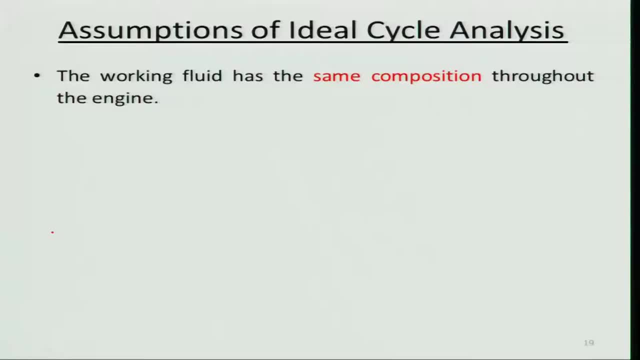 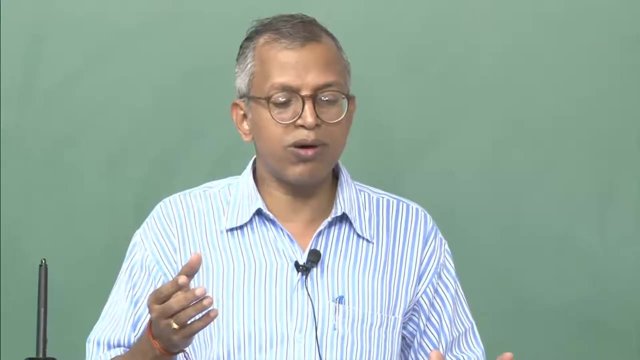 So in the particular we did, The working fluid has the same composition throughout the engine. When I say same composition generally, we take is air. If you look at, whatever the assumption I will be talking about in thermodynamics, known as air standard assumptions, That means you know this. we know that combustors in which you will be adding fuel 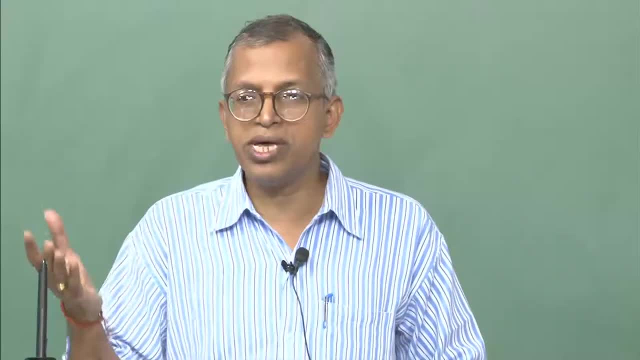 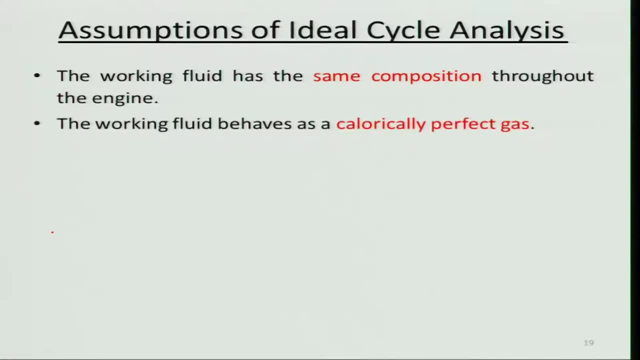 It will be converted into various components, various spaces, But however, you are not considering just for the simplicity sake. And working fluid behaves as a calorifically perfect gas, The perfect gas, you know. Of course, it will be valid all the time because, although the pressure will be high, 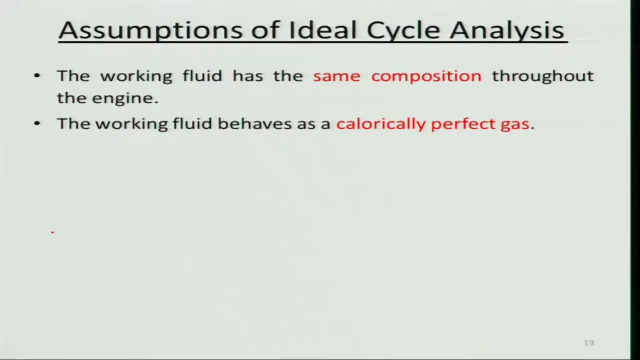 But temperature is being higher. you can do that, But here you are saying calorifically perfect gas, because the properties would be changing, Although the temperature will be changing as you go from various components of a gas turbine engine or a ramjet engine. Of course ramjet engine we will be discussing today. 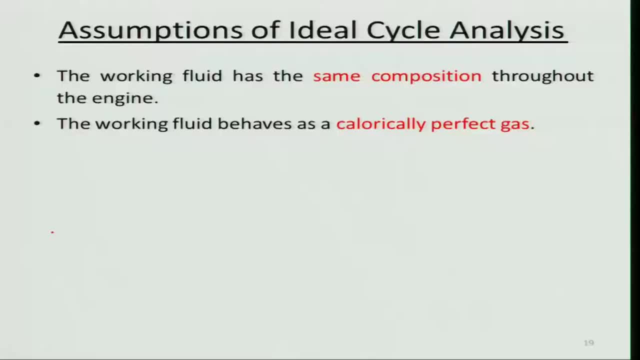 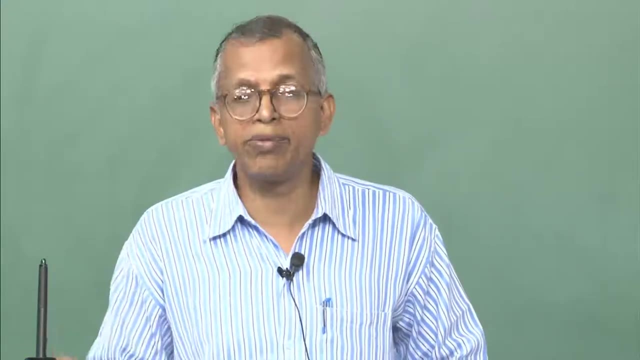 So, but that we are assuming for the simplicity, And fuel flow rate is negligibly small in comparison to air flow rate, Because if you look at the ratio air to fuel flow rate is around 30 kind of things. Of course it can vary from 20 to 40 or even more right. 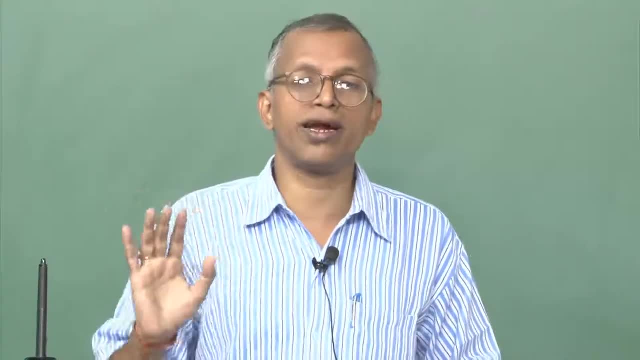 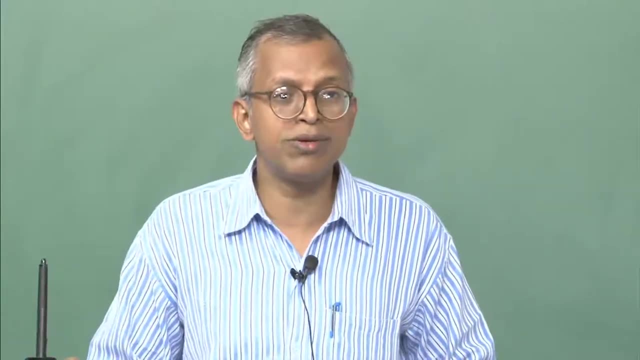 But we are neglecting. Whenever we are comparing, we will neglect, But in other places we would not be neglecting. For example, if I am talking about TSFC, Specific fuel conjunction or thermal efficiency, Can I neglect say that, ok, m dot f will be 0. 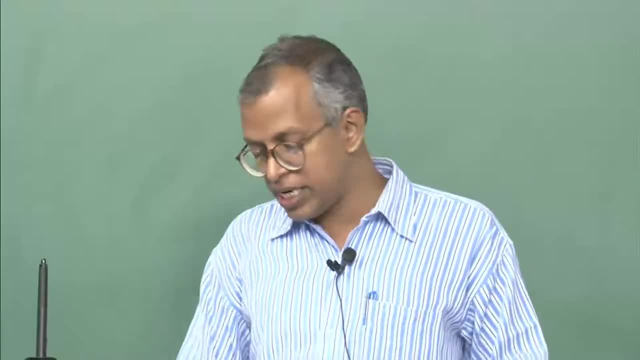 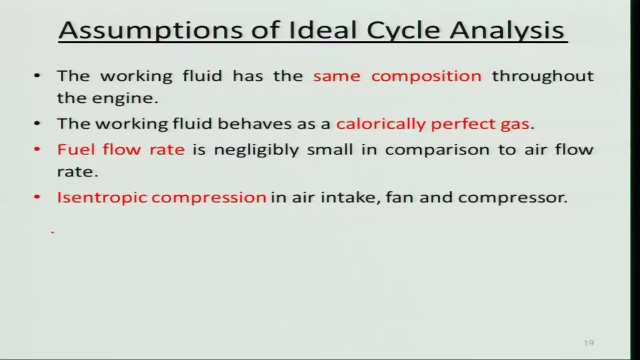 I cannot manage to do that right. So that way you should understand Comparison. whenever we are comparing we will have to neglect And isentropic compression in air intake, fan and compression. So compression process occurs in all these three components. So we are saying isentropic. 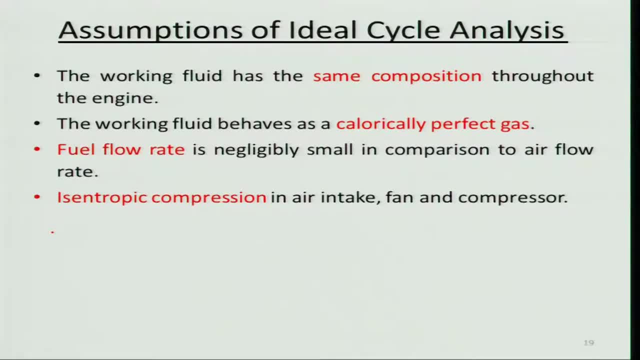 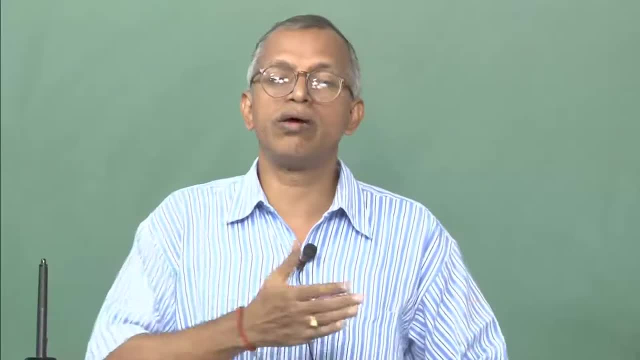 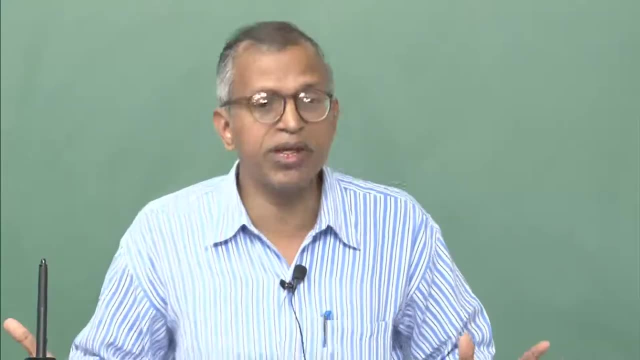 But in real situation it would not be. Isentropic means reversible and adiabatic. How can that possible? It is not possible. Of course one can say that heat- the fluid is flowing through the compressor and air intake very fast- May be heat loss to the ambient will be very low. 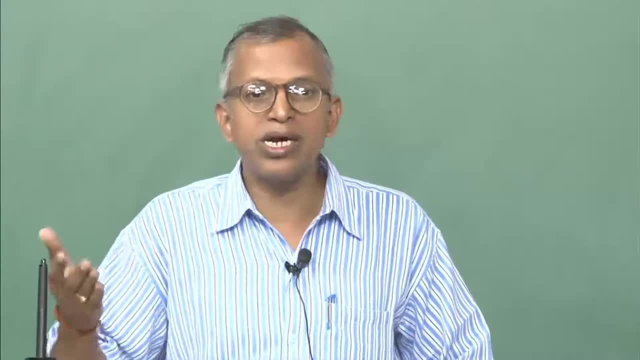 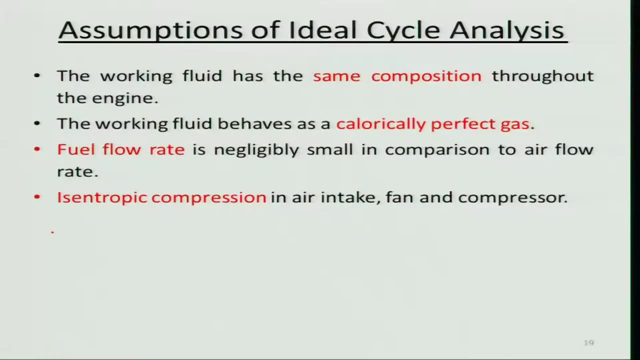 You can neglect it, But it cannot be reversible. Friction will be there. Without that you cannot really do much right, particularly in compression. So therefore you cannot have what we are doing for simplicity And isentropic expansion in turbine and nozzle right. 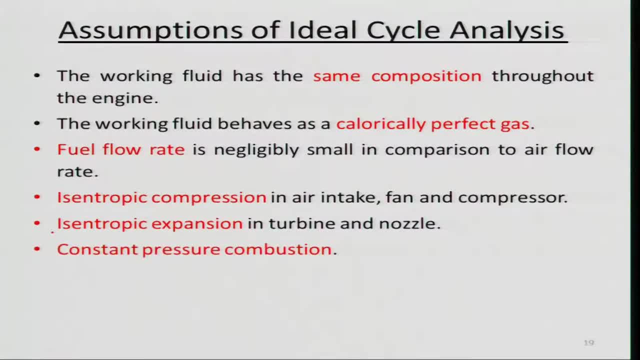 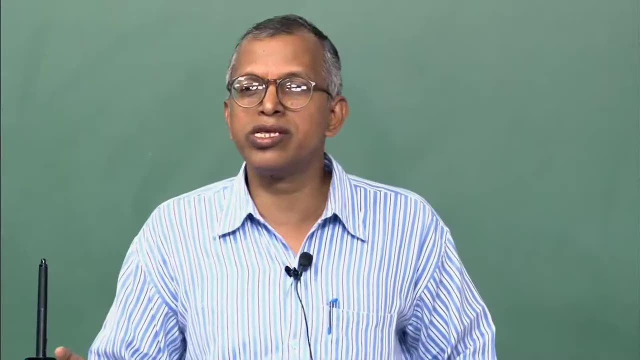 And constant pressure combustion. we are assuming right, Because this is the deflagration And, unlike it, is not a combustion chamber or the close volume where combustion taking place, So here the pressure is remaining constant. One example I always give: as if the combustion is occurring in a well 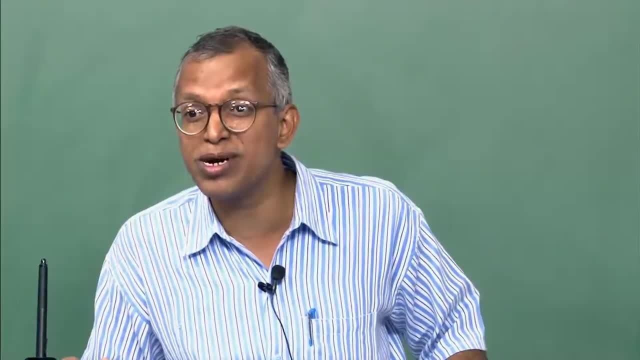 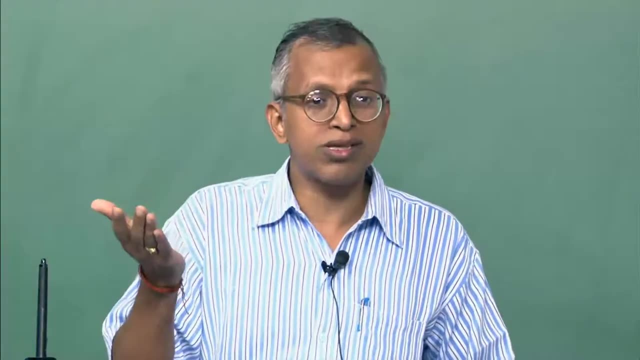 But if it is a close surface, can I say pressure is remaining constant. during combustion It will be increasing, like in your IC engine internal combustion- This model as a constant volume process. We have seen that adiabatic temperature under constant volume and constant pressure will. 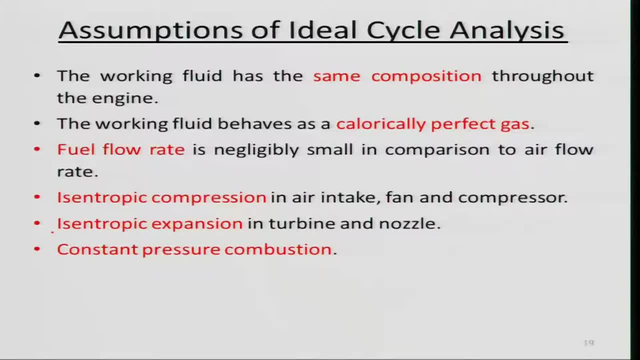 be different, right. So similarly, this is again we are making and it is not that bad. But however, we are also assuming in these the total pressure loss in during the combustion is negligibly small, right, which is not the case. No pressure losses in air intake and combustor nozzle. 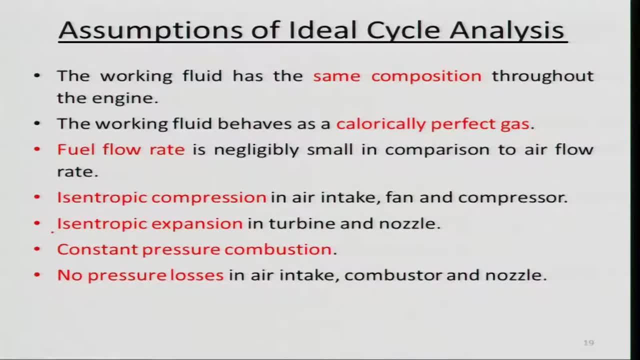 Right, As I told just now, not only combustor but air intake and nozzle. there is no pressure losses. It is not possible in real situation. but we are doing, we are assuming that. But to engine exhaust is expanded fully in the nozzle right. That means it is a what you call. the thrust is contributed due to the momentum. 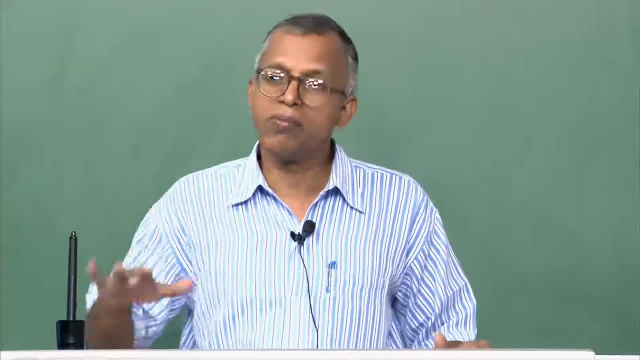 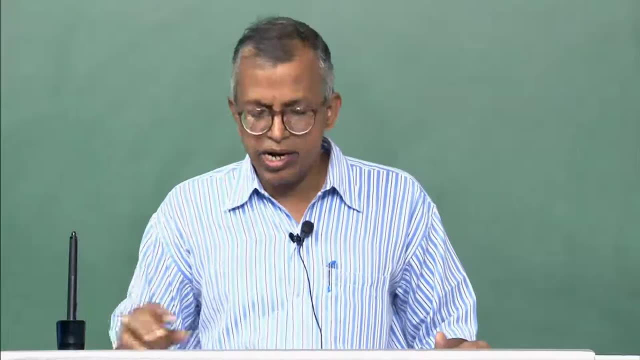 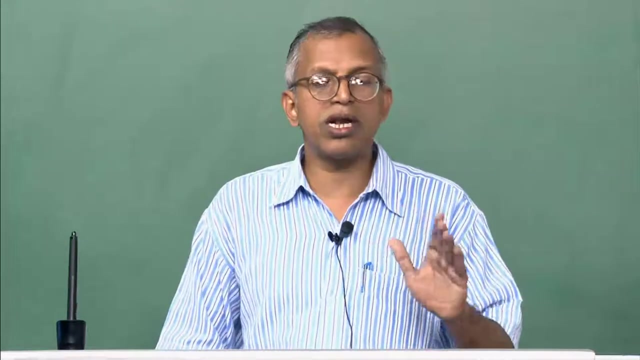 And it is of course that is ideal situation because, particularly in rocket engine, other which we are not considering, But there you cannot have. here you may be, some resume, it will be expanded fully. another resume, it will not be So. with this assumption, now we will be, you know, moving into ramjet engine, keep in mind. 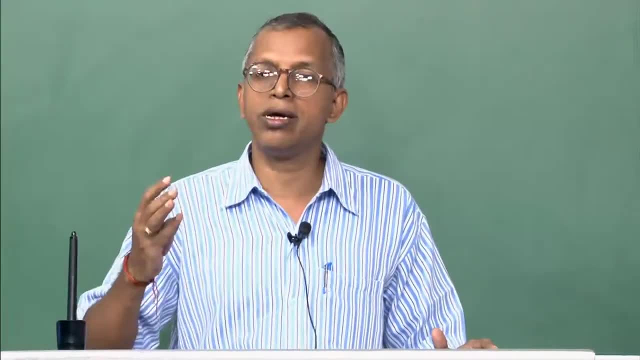 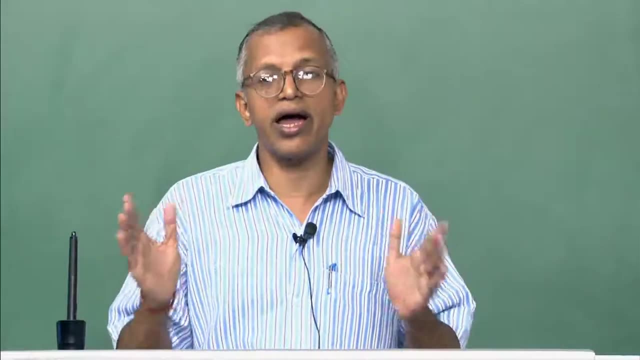 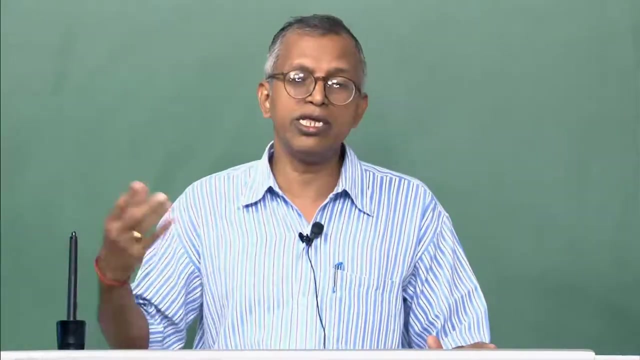 these assumptions will be valid for ramjet and then turbo fan engine, turbo jet engine, turbo prop engine. what we will be discussing under ideal cycle And what we are doing: we are basically looking at parametric cycle. That means we will be varying those parameters and see how it is affecting the various performance. 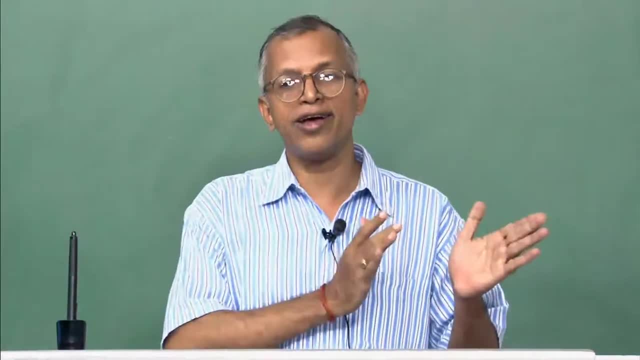 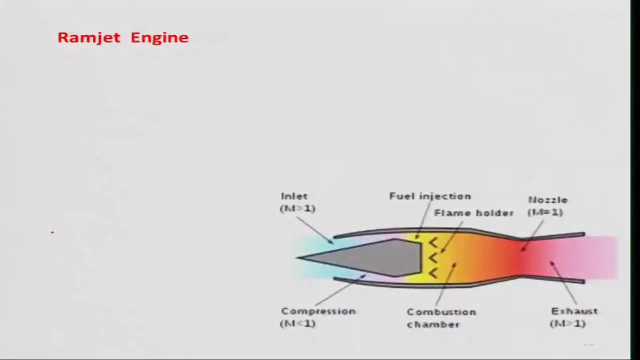 parameter. that is the objective of this cycle analysis, Unlike your other analysis. what you have done that it can be used as a design tool. So let us look at ramjet engine. if you look at a ramjet engine, I have shown a schematic diagram. this is having portion is air intake. 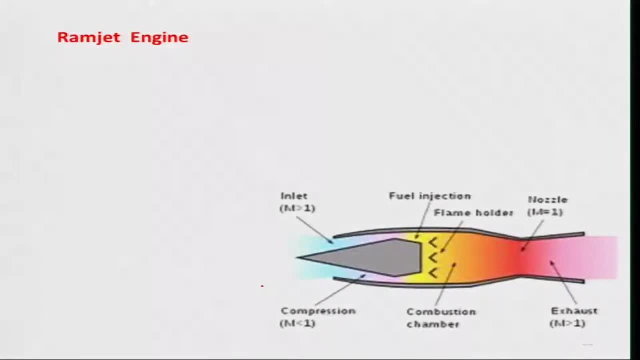 In this case the what you call Air will be entering and from the supersonic speed, because ramjet engine operates under the supersonic speed kind of thing, And it will be entering and then decelerated. that means compression of air will be taking place. 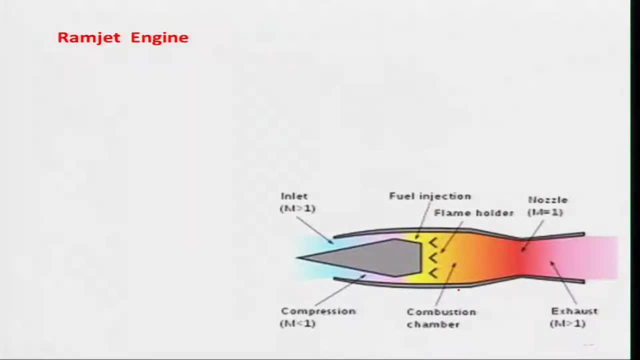 And then it will be burned in the combustors. of course flame holder will be there and once this high temperature, high pressure gas being produced, it will be expanded in a nozzle which is nothing. It is a CD nozzle, conversion diversion nozzle, right. Let us look at actual cut away view of a ramjet engine. why the name ramjet is there? 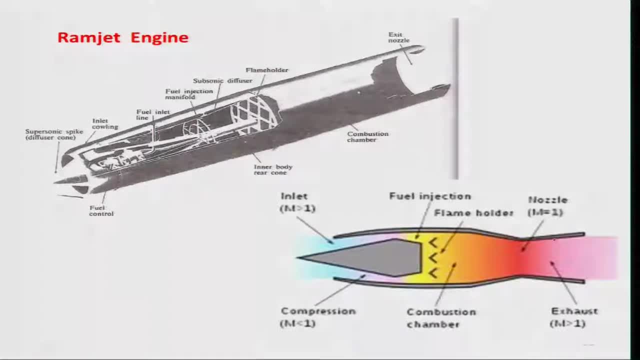 because in this case the ram pressure is being utilized, For example, when the what you call air is coming at a supersonic speed and it will be having a supersonic spike and it will act as a diffuser- What you call this known as supersonic compression- right till that means the air will be decelerated. 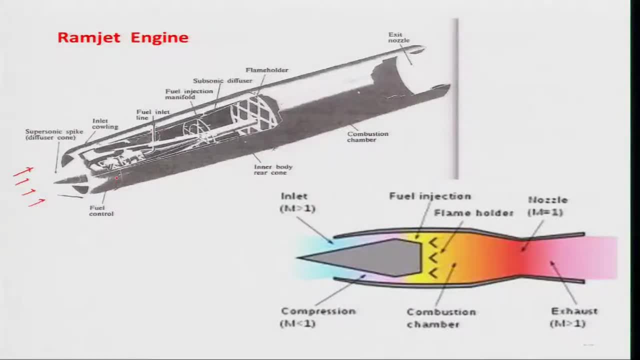 from supersonic speed to the sonic in the what you call in the intake, supersonic intake, and then from sonic to the subsonic. you know it will be taking place. Beside this, you need to have, you know, fuel, because fuel has to be burned right and for 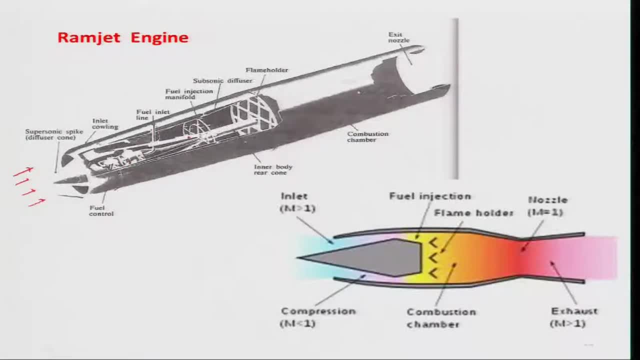 that you need have a pump and then inlet will be there. it is injectors or the atomizers. you know there will be fuel manifold here. fuel will be being stored generally, you know, like in your Boeing aircraft, and the thing where fuel is being stored it is stored in. 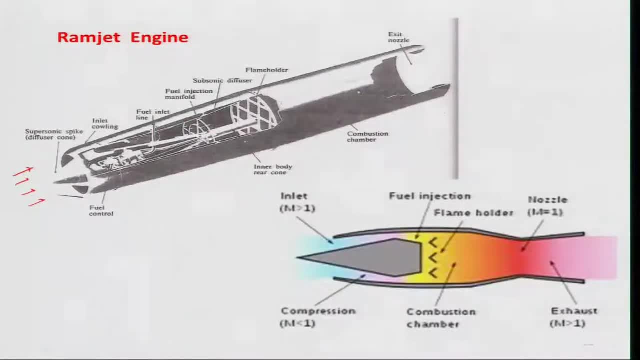 the wing right kind of thing. So therefore, in the fuel injections that atomizers it will be there, and then it will be mixed with incoming air, Incoming air, and it should be good, and then when you burn, the flame has to be you know. 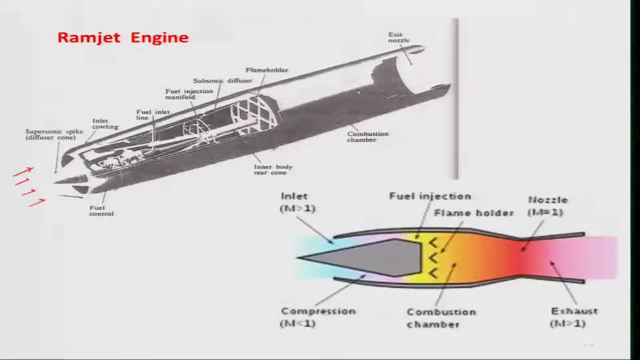 stabilized with the help of flame holders. Very simple stabilizing mechanism is being used and when this hot gas is being produced at a high pressure, it is what you call expanded in nozzle. if you look at, this is the convergent divergent, which is very, very small, you know. in this case, this one. 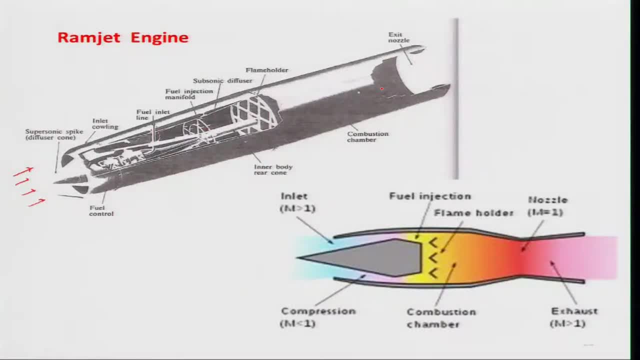 But then what about this thing? Because there the mixing and combustion will be taking place. it will be uniform, So that you know, and combustion will be complete because it is at a little higher speed. and keep in mind that here the subsonic combustion happens, not supersonic combustion. 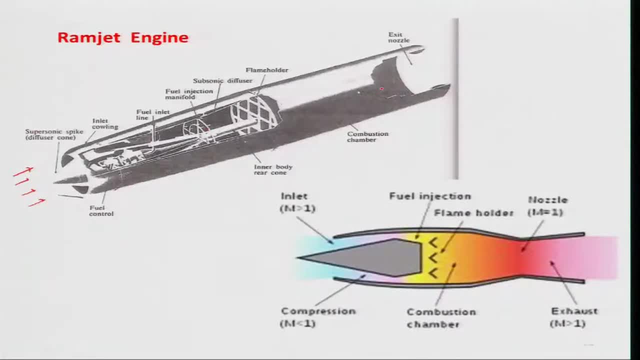 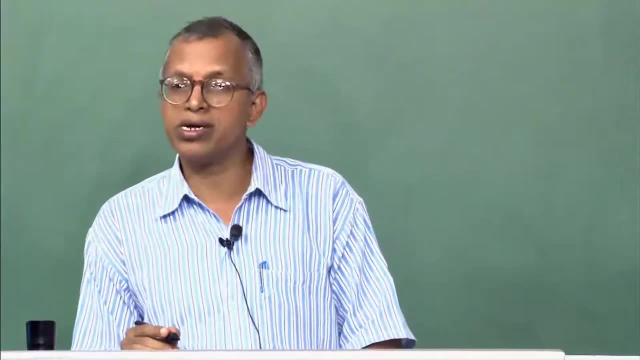 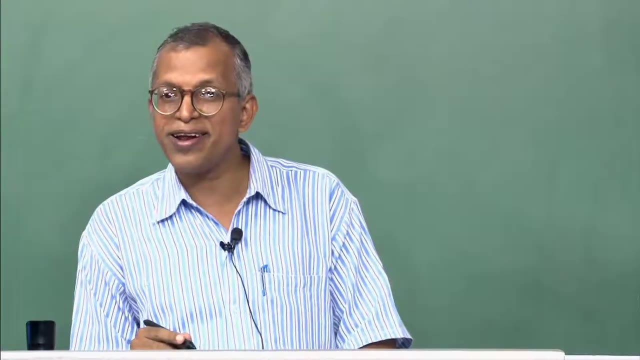 So now, if you look at it, is a quite a simpler system as compared to the gas turbine engine, right, Why? because it is not having compression. if compression is not there, that means it will be not having any turbine, So and there is no sap as such. and then the complexities. you know it is a very, very simple. 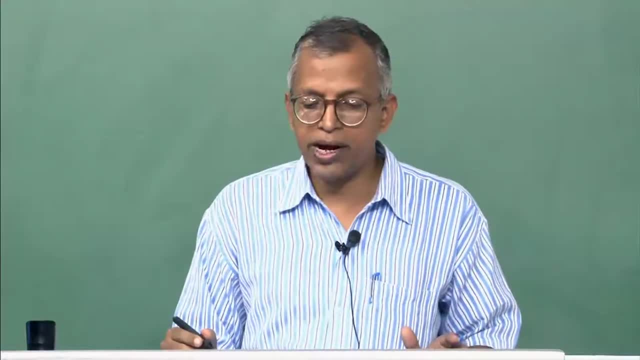 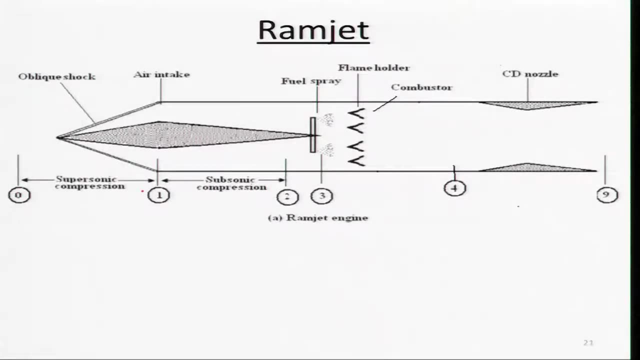 thing. Let us look at a schematic of a ramjet which will be using and keep in mind that 0, we are saying is the station number and 0 to 1 is your supersonic compression and basically it is supersonic. the air has to be decilated from supersonic station. 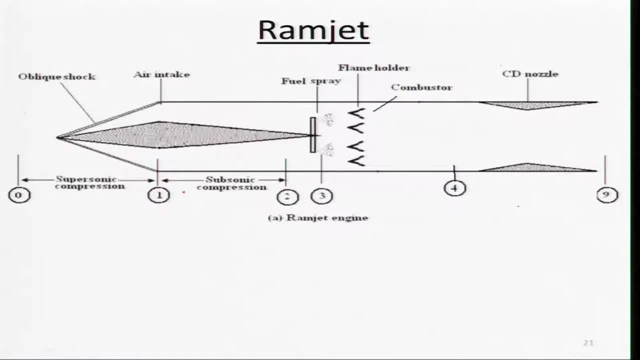 So this is the speed to the sonic condition and then from 1 to 2 is a subsonic compression generally people design for to achieve 0.3 Mach number. Mach number of 0.3 at the station 2 at the exit end of the or exit of the air intake right and the total 0 to 2 is nothing. 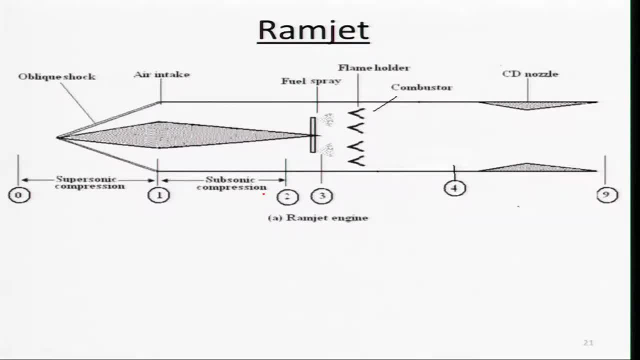 but your air intake, like combined with the combination of both supersonic and subsonic, And then the. of course there is no compression, although we are keeping the same station number. this is a 3, 2 or 3 is almost same, you can say, although it is not shown in this figure. 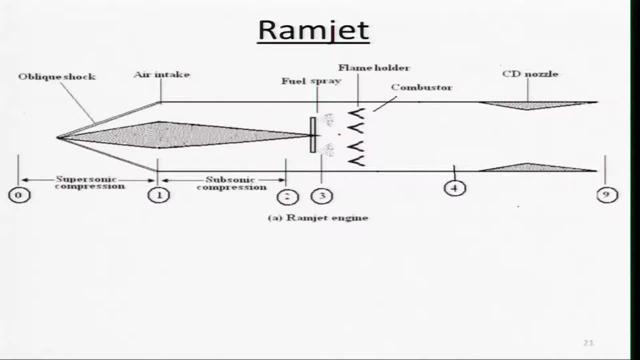 and then 3 to 4 is your combustion, where the fuel will be sprayed and mixed. and then you know, stabilize with the help of flame holders, which are basically gutters, is being used for the flame stabilizer and expanded in nozzle. that is 4 to 9 right. 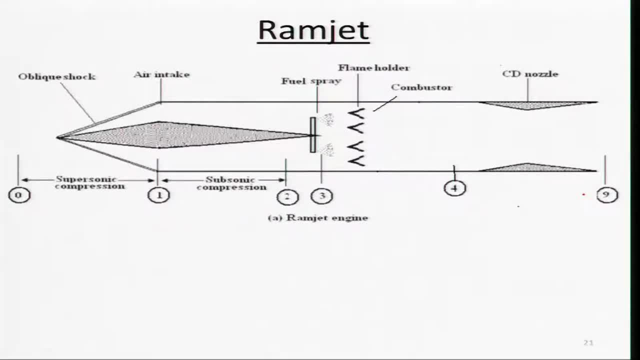 So why we do not need a compression here? because of fact that the air will be entering at a very high speed, for example, if it is entering Mach number around 2.5 right, greater than equal to 2.5 right, or you can say it is equal to 2.5 and we will have to now compress. 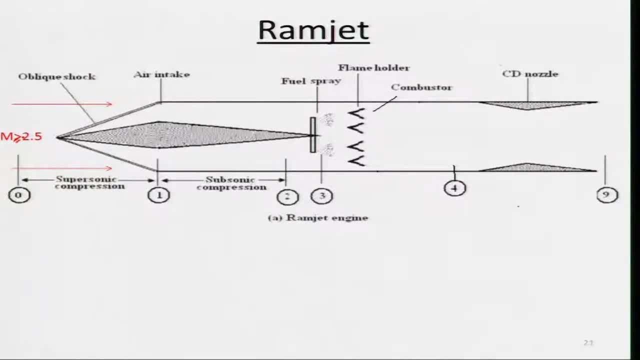 it or decelerated it, you know, because we are compressing by decelerating the flow At the end of the air intake to 0.3, equal to a simple calculations of isentropic flow, you will find the pressure ratio of something around 17- 18 you can get. So then, if I am, 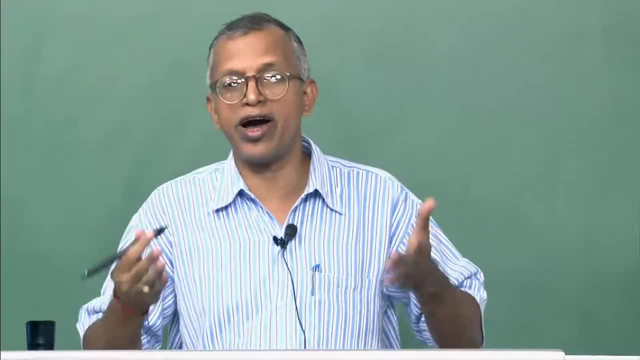 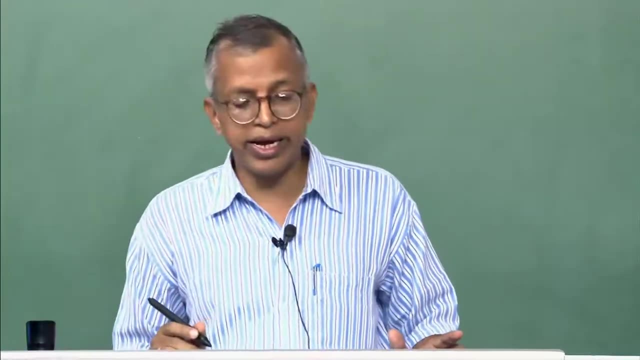 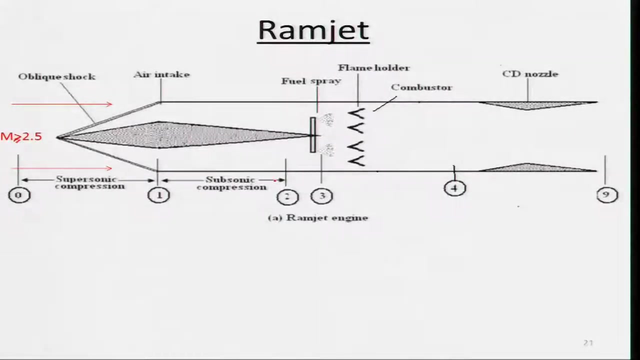 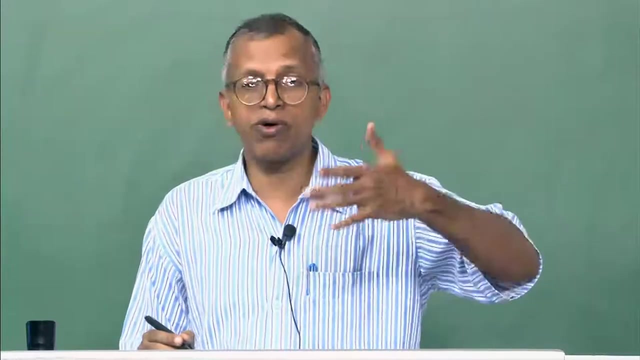 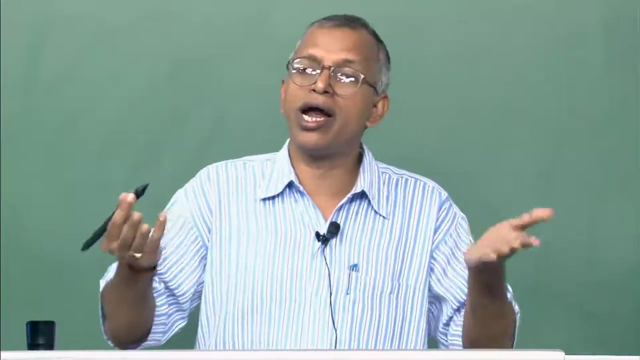 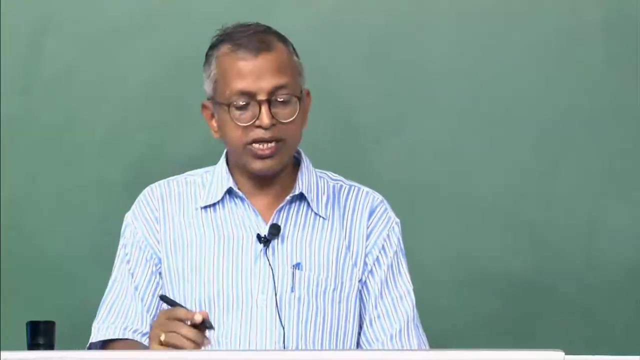 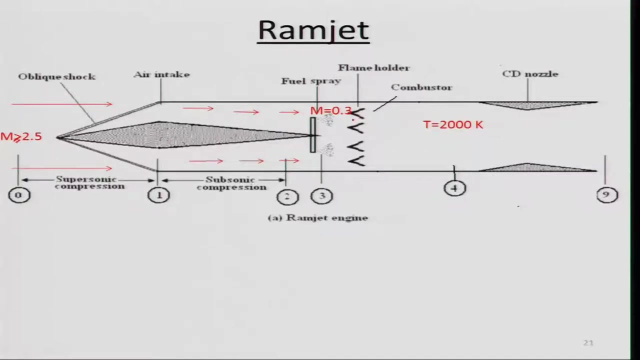 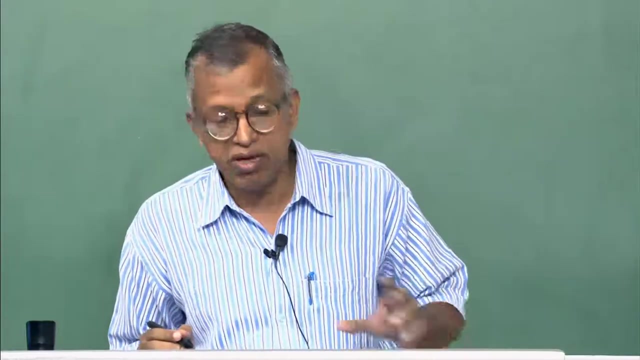 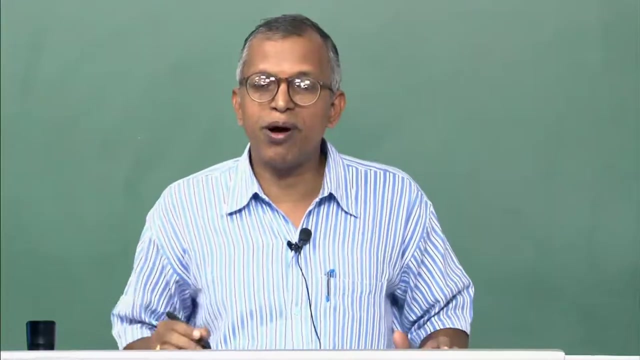 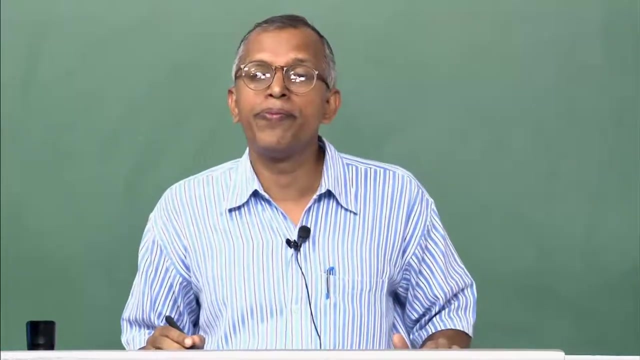 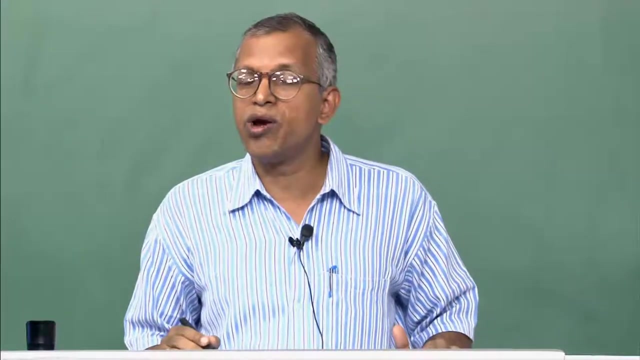 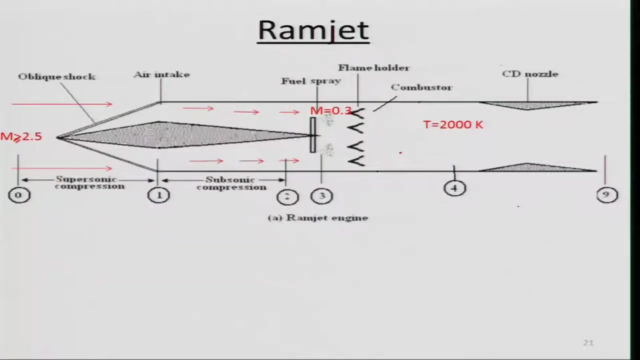 getting a pressure ratio of 18 or 17, you know it is good enough. I need not to really go for a compressor, which is a very bulky and costly affairs. So also the turbine I can. Yes, you know, based on the ram. jet means with a rocket or in an air craft, you know. 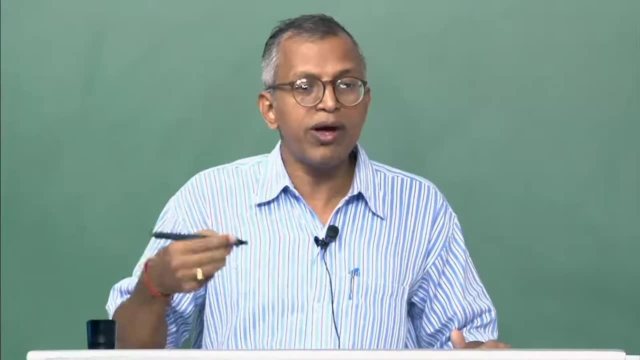 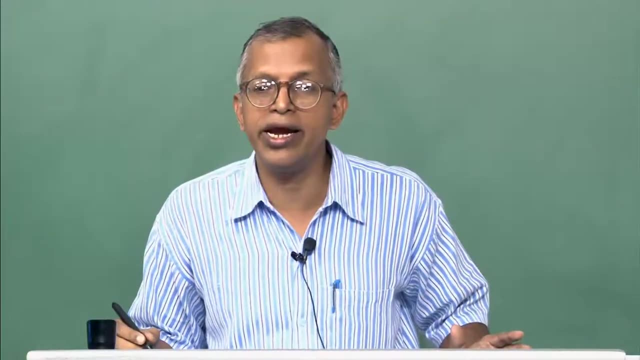 supersonic air craft, fighter air craft, then I will. But if I want to- no, I am not happy with that- I want to use a ram jet from the ground itself. What I allowed to do. What are the ideas? can anybody tell me? 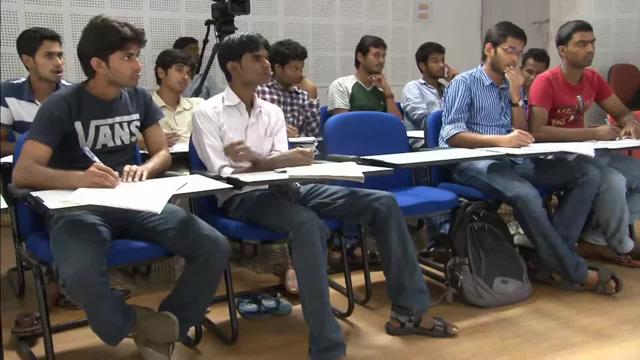 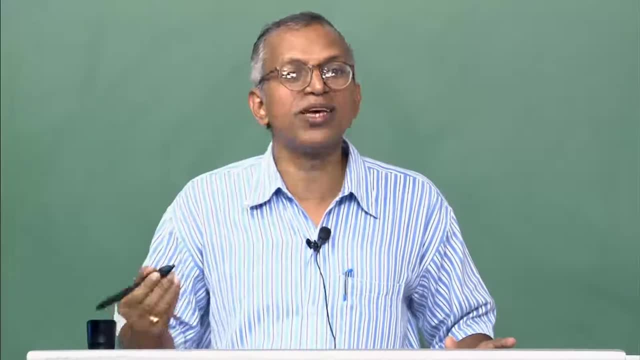 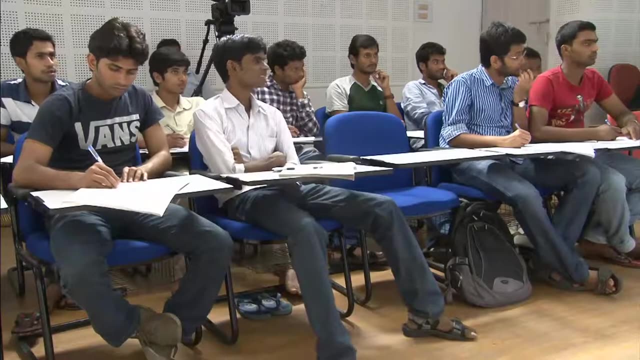 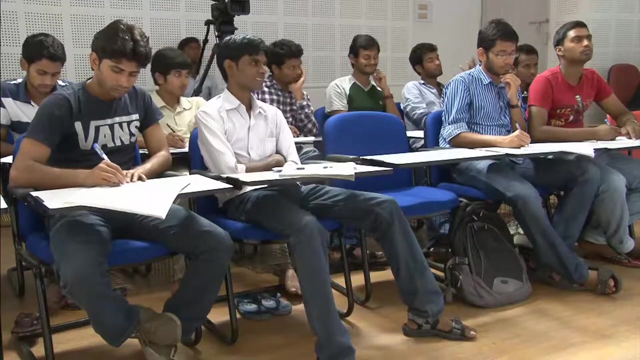 Pulse jet, Hmm, Pulse jet. Pulse jet itself I can use. why should I use ram jet right Rocket? Roger RotRight Rocket is already being used. but I want to do something. so what I will have to do, So what I am thinking. I will leave this question to you and think about it, if you come up some. 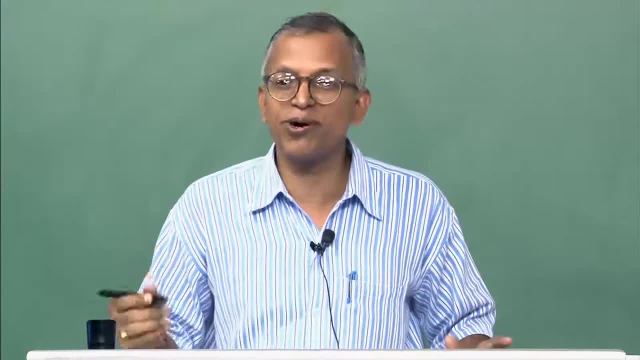 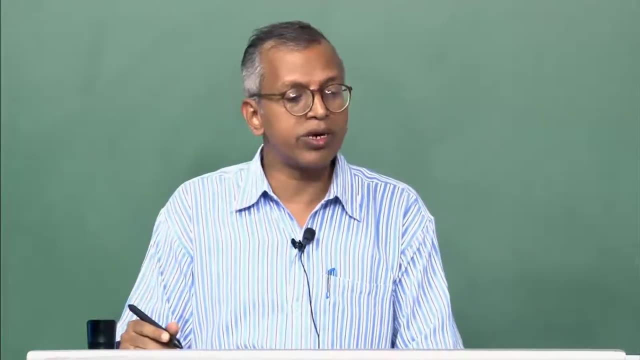 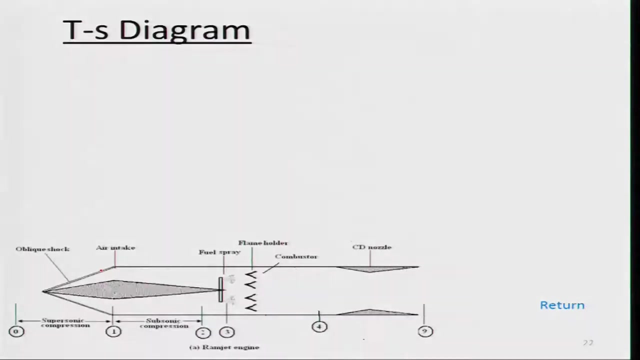 ideas without looking at existing one, then you know it will be interesting to discuss. Otherwise, some ideas I can give I do not want to give at this moment, later on we will see. So let us look at how. what are the processes are involved. as you told that 0 to 2 is basically. 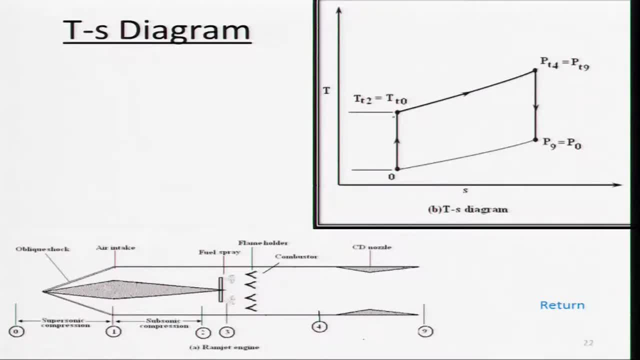 the compression. in a t s diagram I can write down 0 to 2, that is the compression right, isentropic process, isentropic compression. But if I look at in a p v diagram how it will be, compression process: 0 to 2, t, 2 t, 1.. 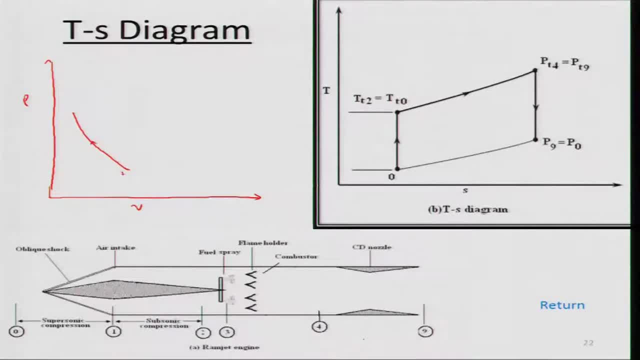 It will be t 2 right and then t t 2 from this station to what you call 4. it is the compression that is constant pressure Combustion right. this is compression Combustion right. this is compression Combustion right. this is compression. 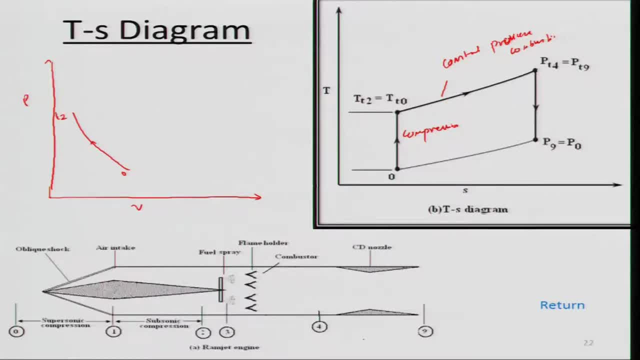 So if I look at in p v diagram it will be very simple. that is a constant pressure, pressure is not remaining constant- and p t 4 to p 9 it will be expansion- expansion where expansion in a nozzle, that is isentropic expansion. So my it will be t t 4 and this station is 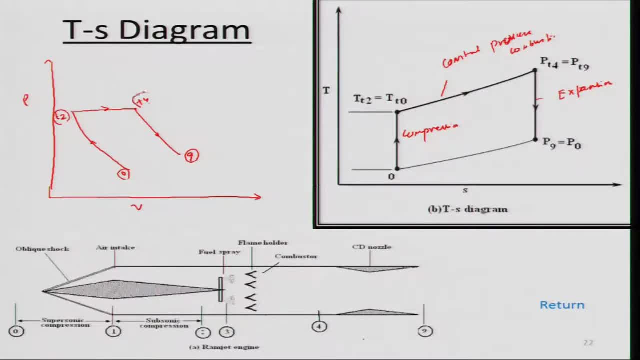 basically 9.. So, and I am just saying it is basically 4 station, we can say, because total we are talking about, totally keep in mind whenever I am talking about ratio in combustion chamber what I will be saying: it will be pi v will be p t 4 by p t 2, right? 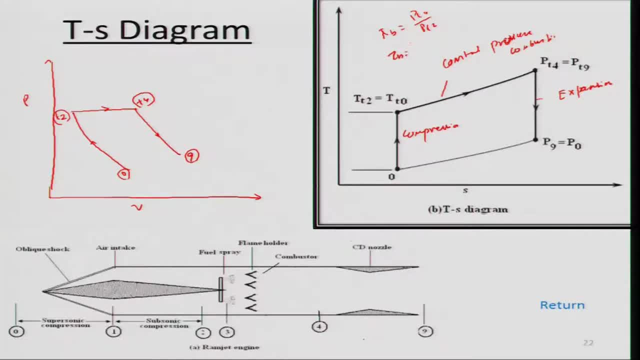 total I am considering, If I say it is tau v, it will be similar t T 4 by T 82. But whereas when I am coming over here it is the static condition, at the exit of the nozzle, at the inlet it is also static and keep this in mind very important. 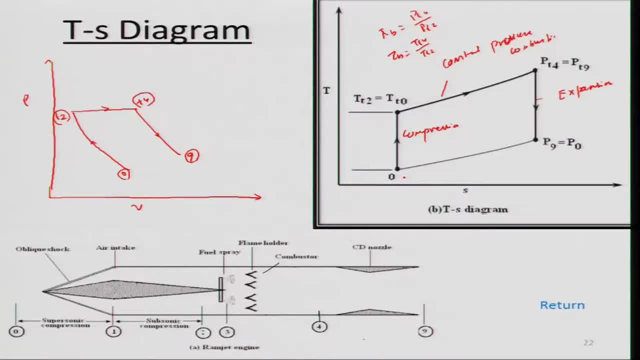 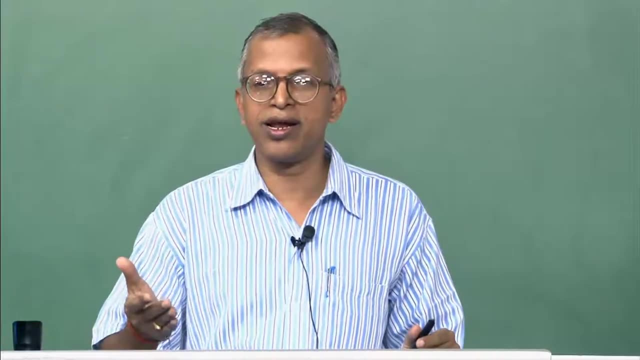 point. So we will be using those things and see that whether we can, you know, use with how we can use this thing for our analysis. Is that clear, any doubt in this? because it is a very important things and we will be using similar stuff. you know, processes describing 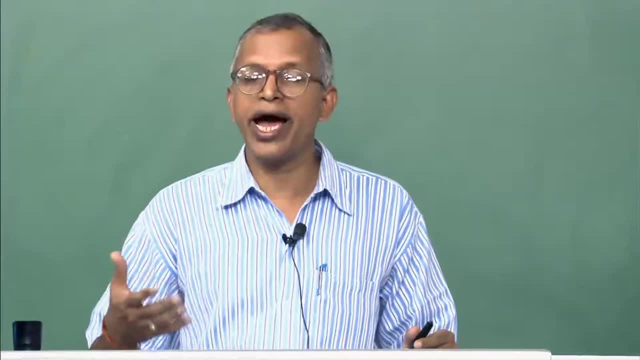 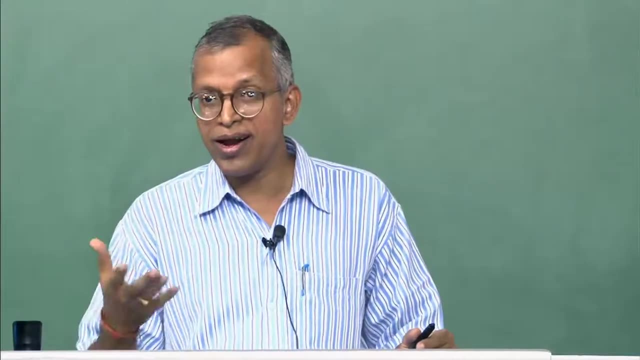 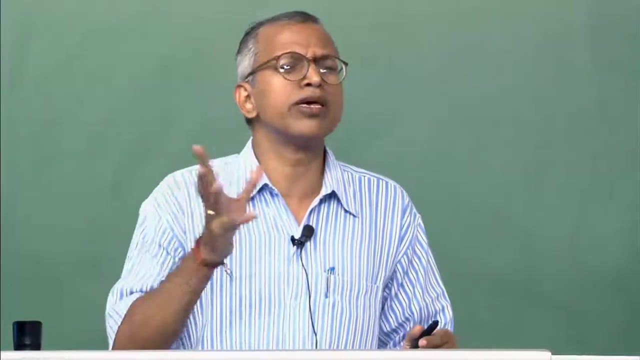 in the process diagram, like T S, P, V. I can have H S. I can have some other thing as well. I can have T V. So you should think about this: how I can, you know, describe the processes in various ways, because that will help you to enrich your mind. 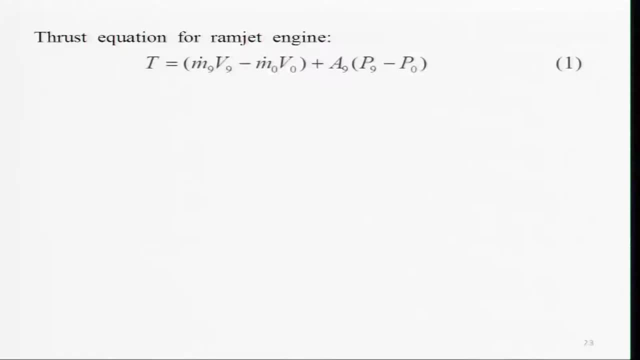 Now the thrust equation for ramjet engine is basically is: the thrust is equal to m dot 9 V 9 minus m dot. m dot naught, V naught plus a 9 P 9 minus P naught. and keep in mind that 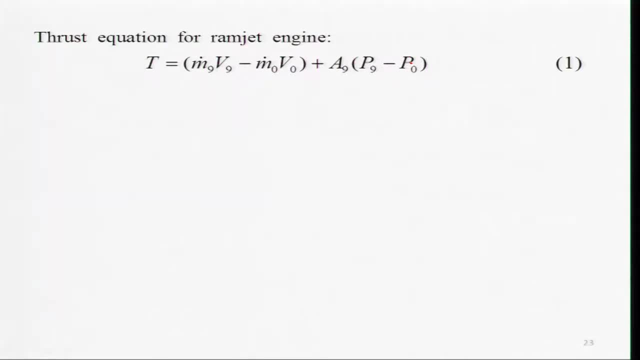 what we are assuming. in ideal cycle it is an fully expanded nozzle. So therefore P 9 is equal to P 9 is equal to P naught, So therefore it is thrust is equal to m dot, V 9 minus m naught. V naught only contributed from the momentum. What we are trying to 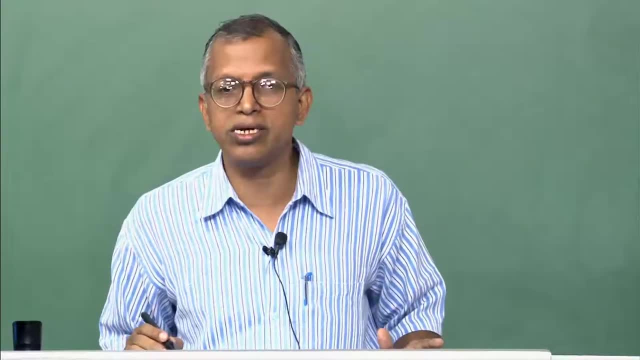 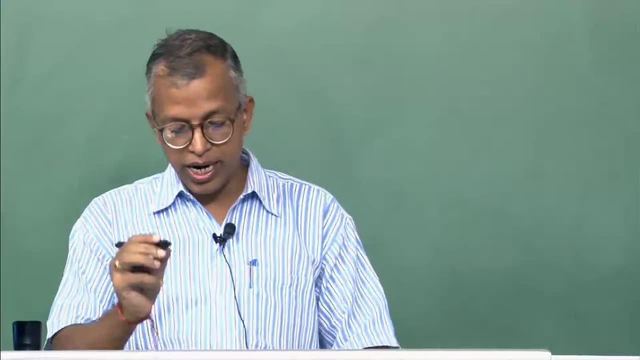 do? We are trying to now express these equations in terms of various ratios So that we can vary and see what we are doing. that is, you should keep in mind, it is involves lot of algebra. So, and as I told, it is P 9, P naught, and then m naught 9 is equal to P naught P. 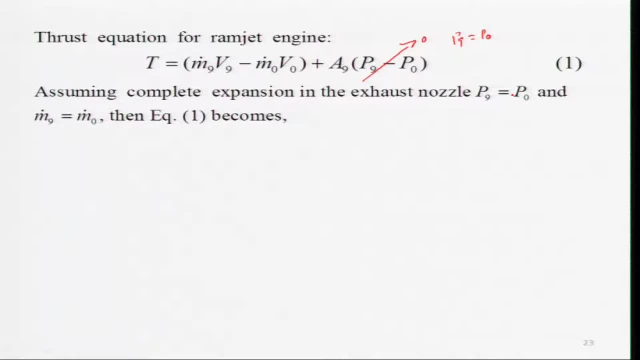 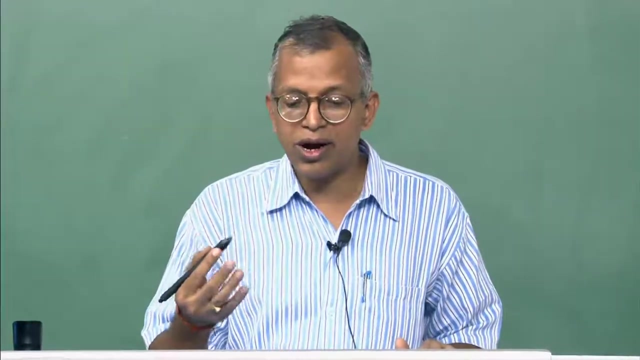 naught, So this is equal to m naught, that we are assuming. that means whatever the mass is exiting, it is whatever the equal to mass is entering. that means we are neglecting the mass of well being added, which is not a you know right thing. but we are doing, for simplicity, What? 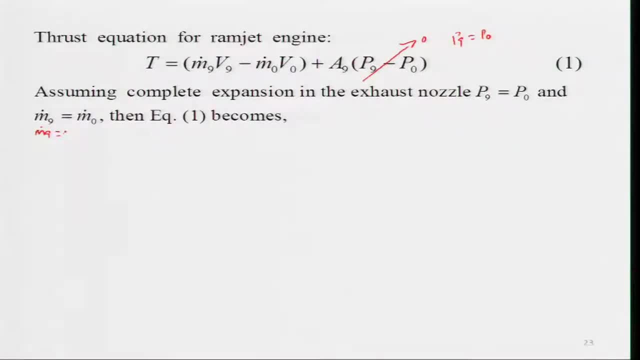 I am saying may be, I can write down here: m naught 9 is equal to m naught naught plus m dot f. So it is small as compare to m naught. that is why it neglect right. So is equal to: 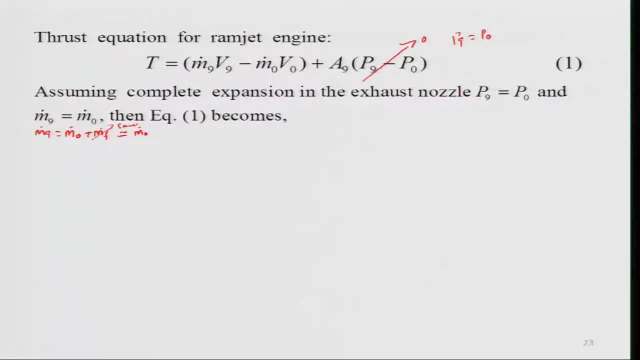 m naught. approximate is not 2.. So what I will do. I can write down this expression. I will take this m naught 9 and a naught, then I am getting V 9 by a naught, right, What I will do. 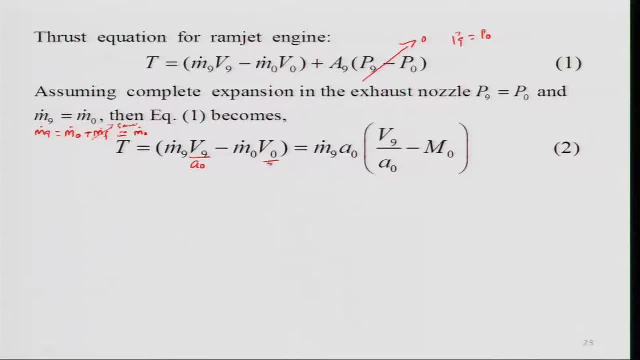 find out this a naught, a naught right, a naught here. So this is nothing but your m naught right, and what we will do. if you look at m? a naught is the speed of sound, right is it? this is the speed of sound, sound where Ambient. 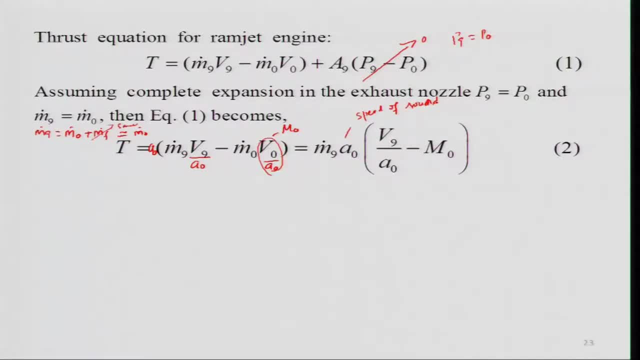 Ambient or the free stream right, free stream speed and m naught is the free stream Mach number. free stream Mach number and this, a naught, is nothing but root over gamma r t naught right, You can, in some place you can see this is gamma naught corresponding to the your which. 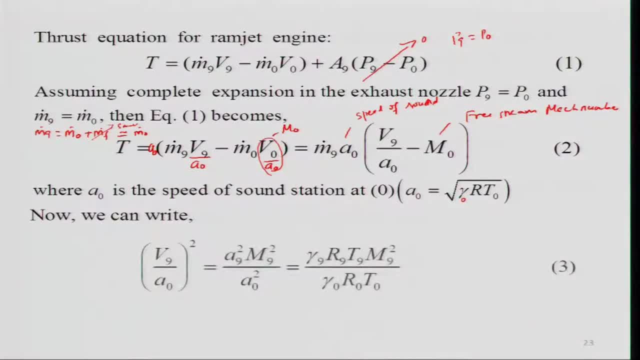 will be using, not in ideal cycle, but in the real cycle. So I can write down: v? nine by a naught whole square is equal to, by definition, a nine square. m nine square divided by a naught square, and this a nine square is nothing but gamma: nine, r, nine, t nine, and we are assuming. 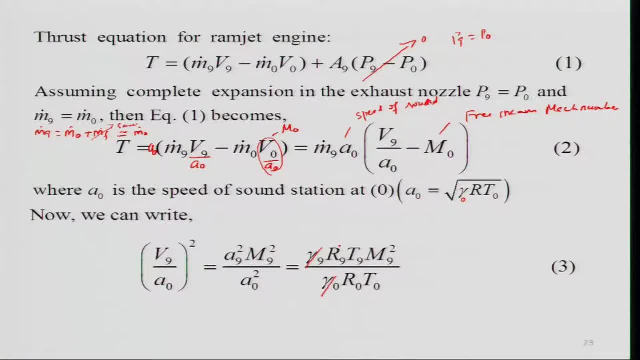 this gamma nine, So v nine equal to the gamma naught, and r nine is same as that r naught. So what we will be getting is right is basically t nine by t naught m nine square. that is right, So 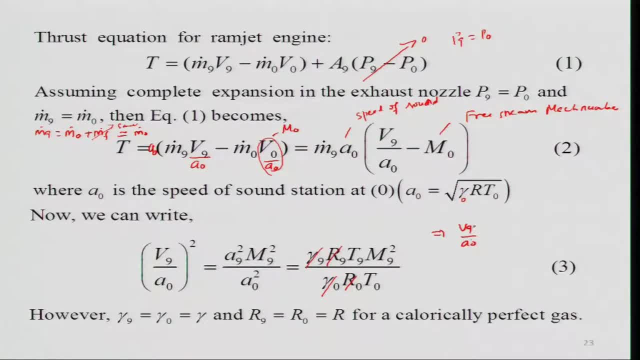 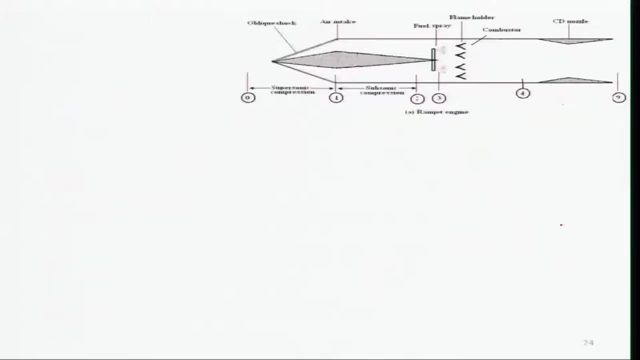 if you look at I am getting here, v nine by a naught whole square is equal to t nine by t naught m nine square. I will be writing the same thing in the in the next line, So is that clear? So an equation three becomes v nine by a naught whole square equal. 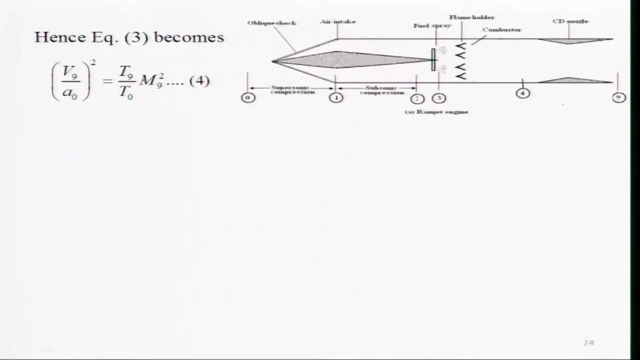 to t nine by t naught m nine square. So if you look at m nine square, I can express for isentropic process right for the, because the expansion is taking place in the nozzle. can I not write down what will be the m nine in terms of pressure ratio? 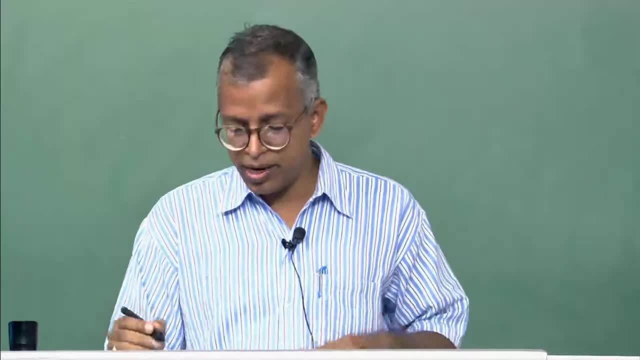 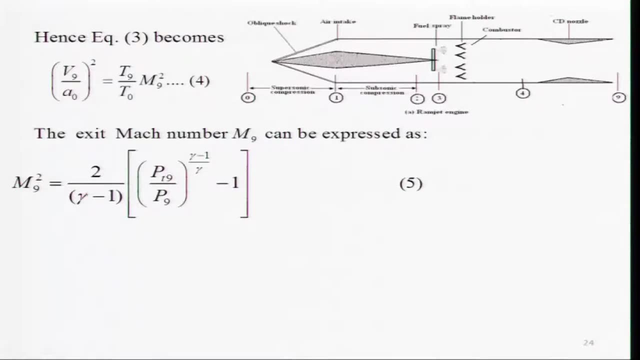 So I am using isentropic relationship, right? So I can write down that m nine square is nothing but two divided by gamma minus one. p t nine by p nine, power to the gamma minus one divided by gamma minus one. this is from the isentropic relationship for the p t nine. 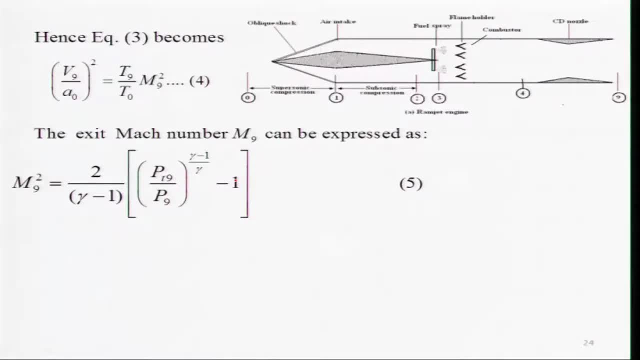 by p nine, p nine, right, nothing, I have just rewritten, right. So what we will do now is we will have to basically look at this p t nine by p nine how it is. you know how we can express in terms of various pressure ratios. So p t nine by nine can be expressed in terms: 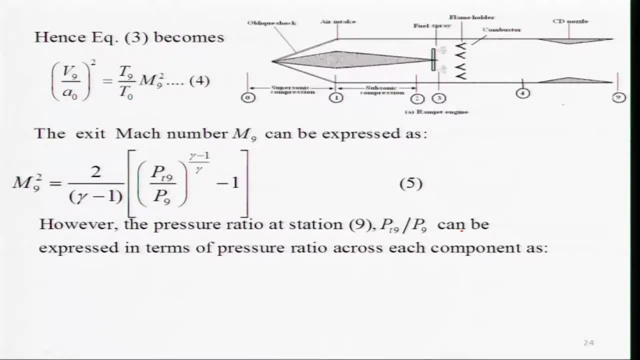 of pressure ratio across each component. what I will do. I can write down: p t nine by p nine is equal to p t nine by p t. four into p t. four by p t. two into p t. two by p t naught. 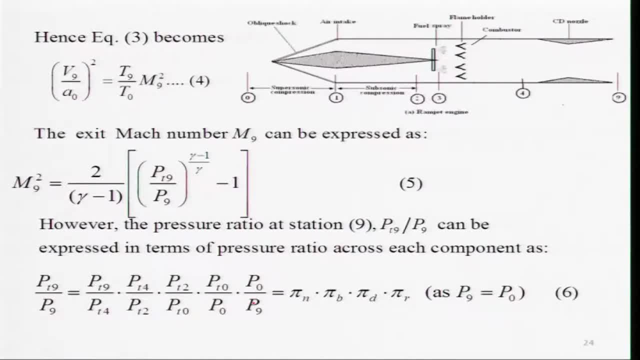 And this is equal to one. why? because p nine is equal to p. naught fully expanded what we have done. So if you look at, what is this one, this is nothing but your pi? n. the pressure ratio is the nozzle. total pressure ratio is the nozzle, and this is nothing but your pi. 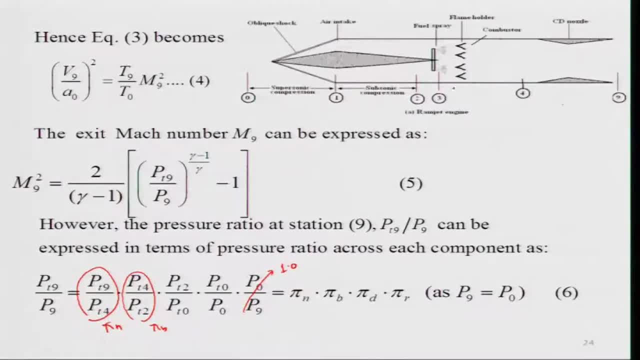 b p? t four by two. this is the combustors right and this is nothing but your pi? d and this is nothing but your pi? r. keep in mind that this is p? t naught. by p naught, that means total right to the static. that is why it is saying it is pi? r by definition, of course. 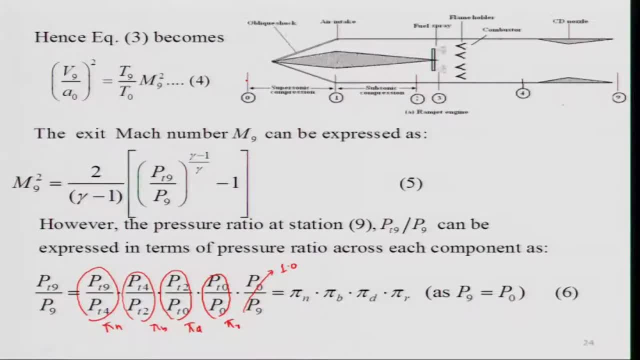 you know, because I have defined that thing, you know next to it. Now what we will do. now we are saying this pressure, that means the Mach number, exit Mach number will be dependent on this pressure ratios. you are getting one, but now it is. 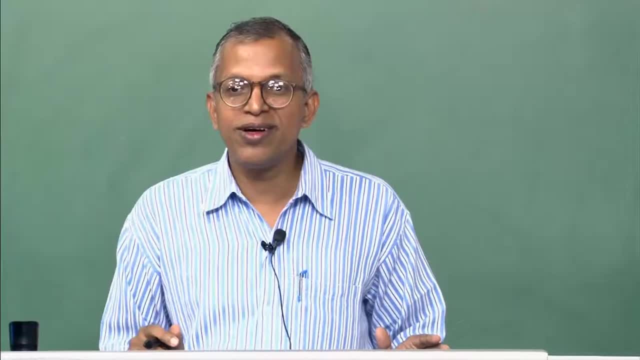 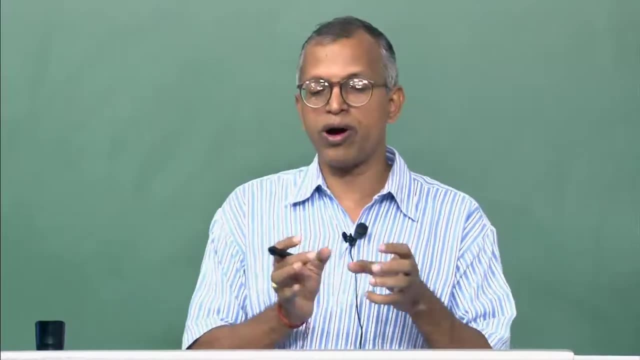 you know too many right, yes or no. And the same thing we will be doing for turbo z, turbo fan, turbo prop- also right, because we are now looking at each component, how they will be affecting the exit velocity, as exit velocity will be affecting the thrust. 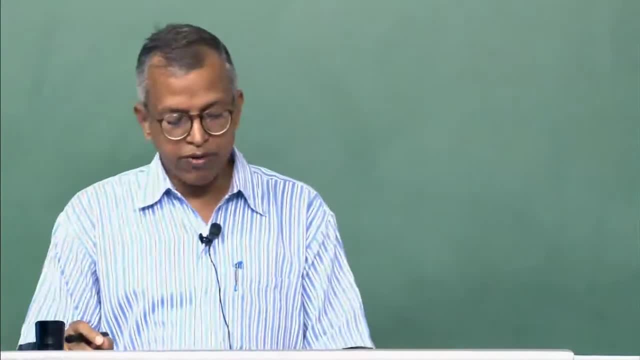 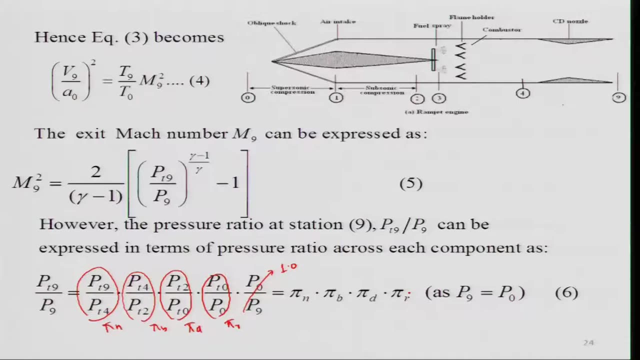 So let us, and if you look at what is this pi n by the, by your assumption, pi n will be one or not. total pressure ratio across the nozzle is is one because there is no loss. so pi n will be one. So what about this pi b, that is also one burner. pi d, isentropic compression. So therefore, 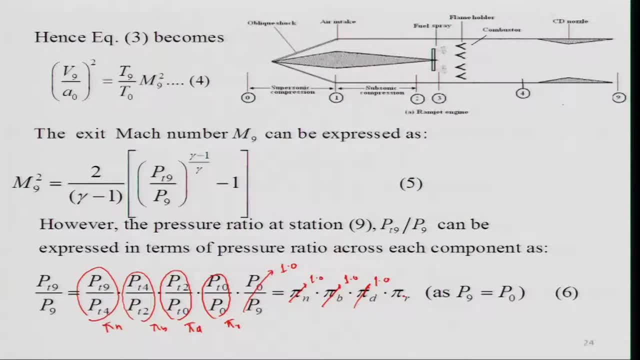 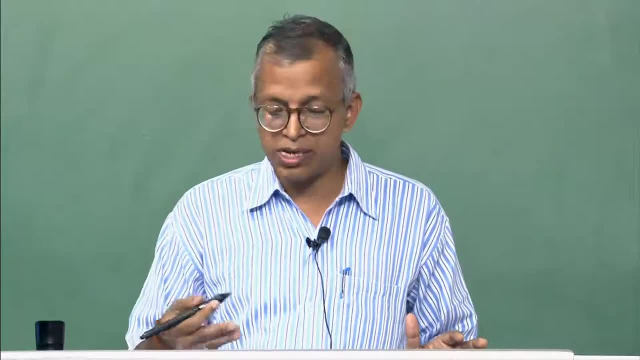 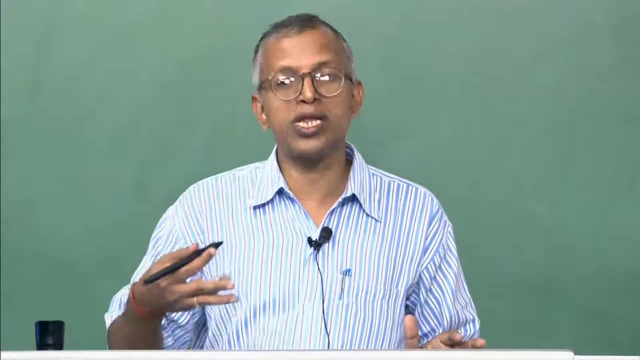 it will be one. can I say pi r is equal to one? can I say I cannot, because Mach number, you know, it is not total. it is basically, except all this thing, pressure ratio. this was the pressure ratio which is with respect to static. So this is nothing but your what you call. 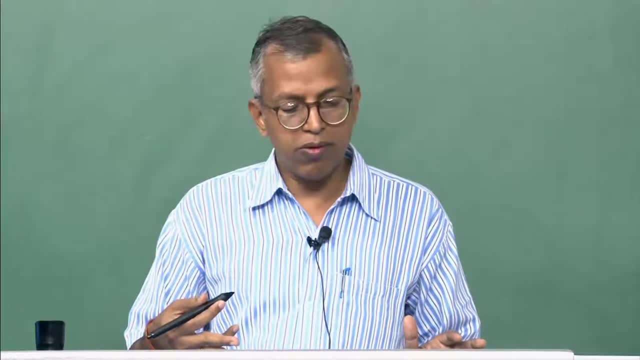 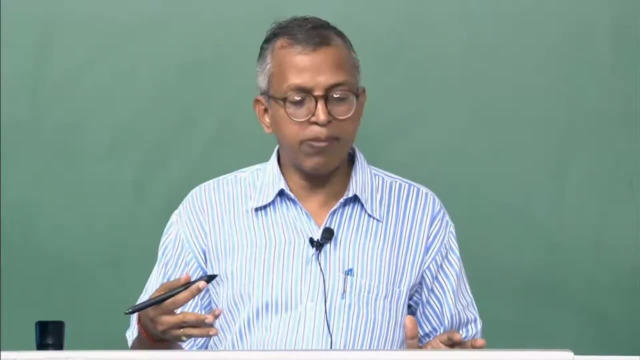 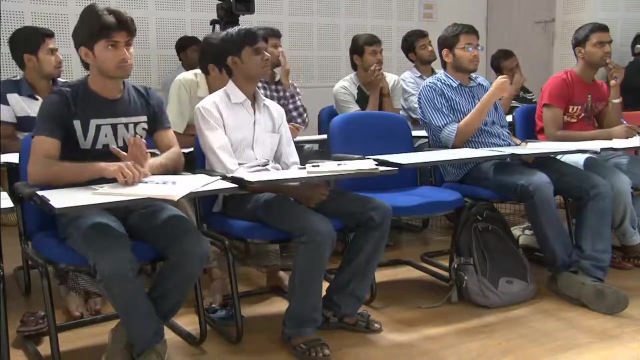 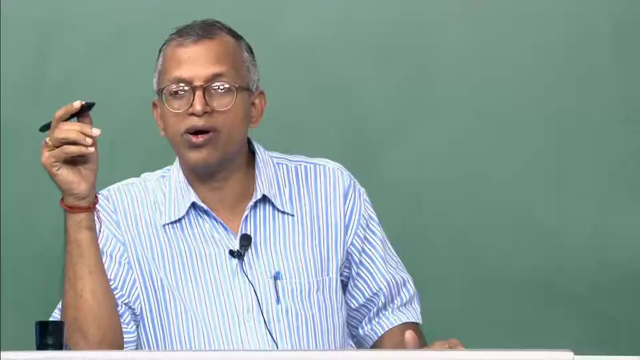 1 minus gamma minus 1, divided by 2 p t by p 9, right, no, sorry, m 9, square, right that one. So that is the assumption we have made. you look at your assumptions. we have looked at the total pressure ratio across the combustor will be zero. 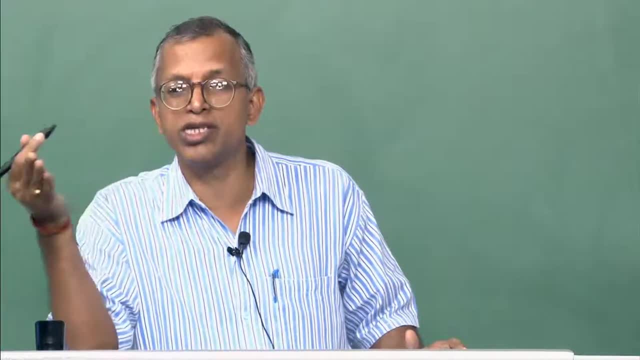 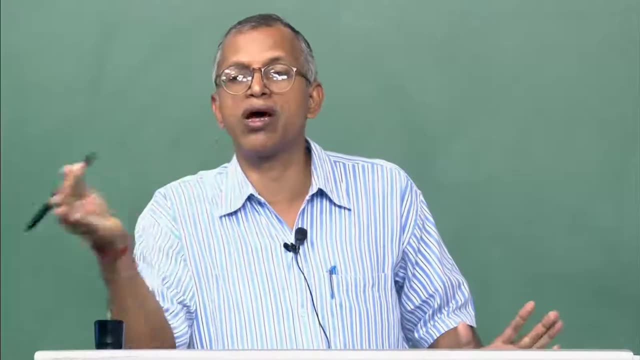 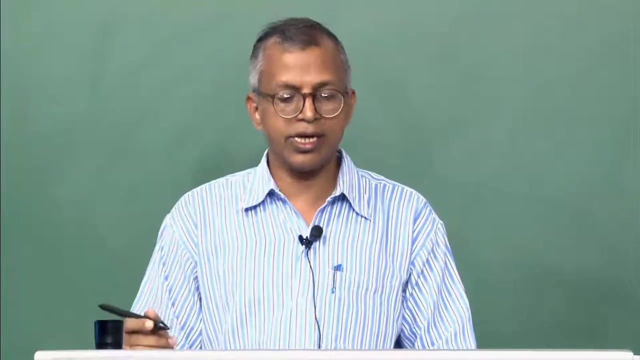 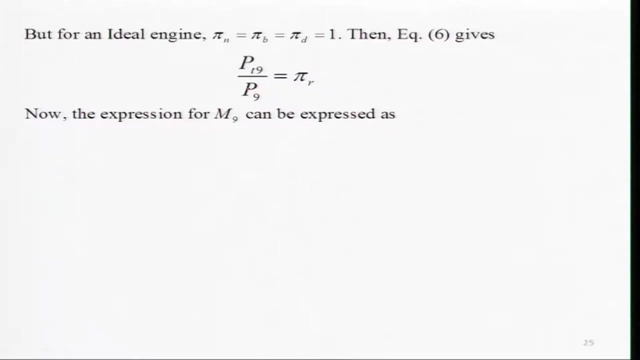 Total pressure loss. if total pressure loss is 0, then p t 9 divided by p t 2 will be one: no pressure losses, right. but however real situation it would, ideal situation it is yes, So what we will do. we are getting pi n pi, p pi d is equal to 1.. So p t 9 by p 9 is 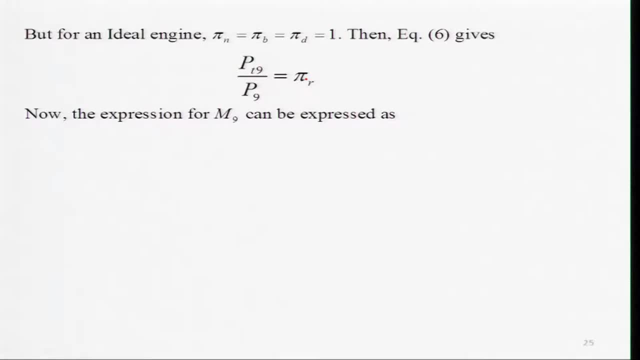 equal to pi r right. And now expression of m 9 can be expressed. as you know, m 9 is equal to divided by gamma minus 1, p t 9 by p 9, gamma minus 1, gamma minus 1.. So what will say? this is nothing but your. 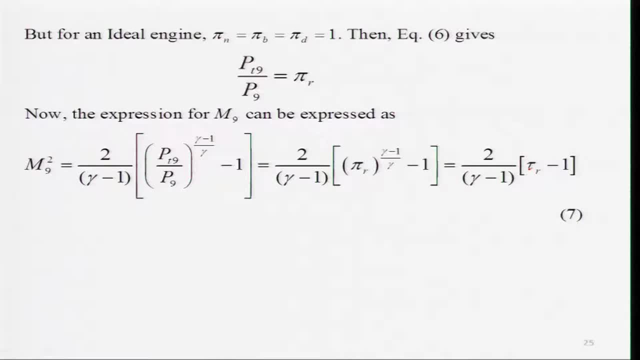 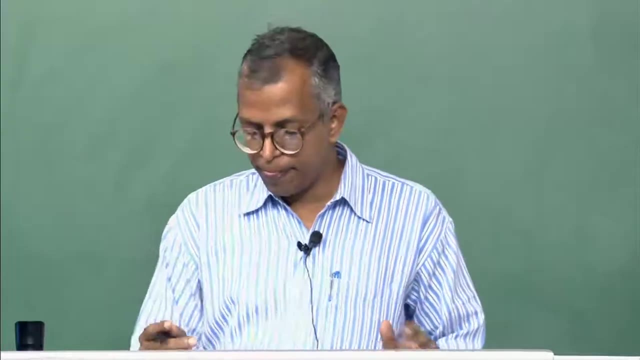 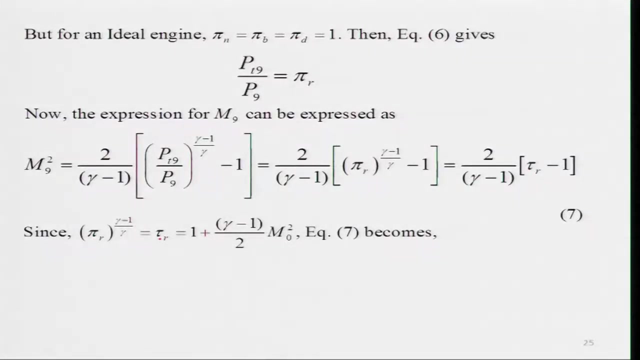 pi r. if you look at pi r, power to the gamma minus 1 is nothing but your tau r, yes or no, because I can relate this isentropic temperature ratio to pressure ratio. isentropic temperature, Right, we know those expression. So therefore. but whereas the pi r gamma tau r is nothing, 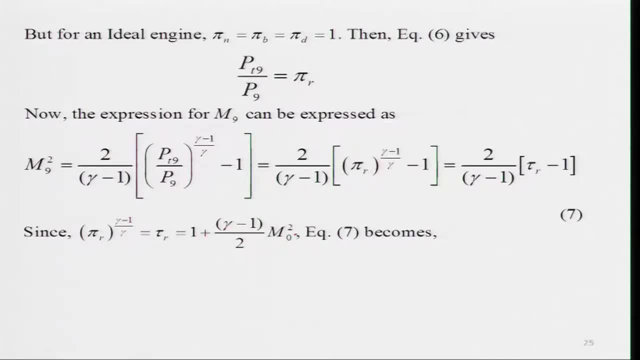 but 1 plus gamma minus 1 divided by 2 m naught square. If I will substitute over here what I will get, I will get gamma minus 1 to m naught square minus 1.. So this will cancel it out right. 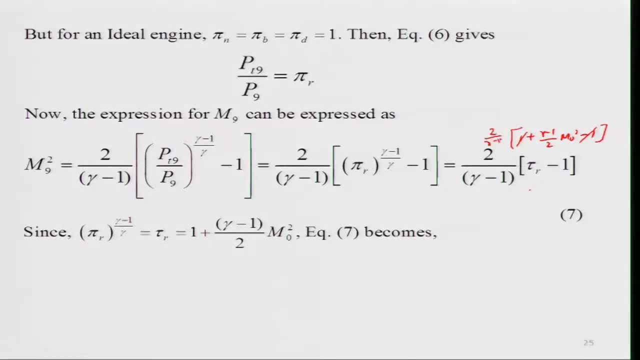 I will get this also will be cancelling out. So 2 to cancel it out is equal to m naught square. what is saying is saying: it is a very interesting statement is saying the exit Mach number for an ideal ramjet engine is equal to the flight Mach number. That means what? 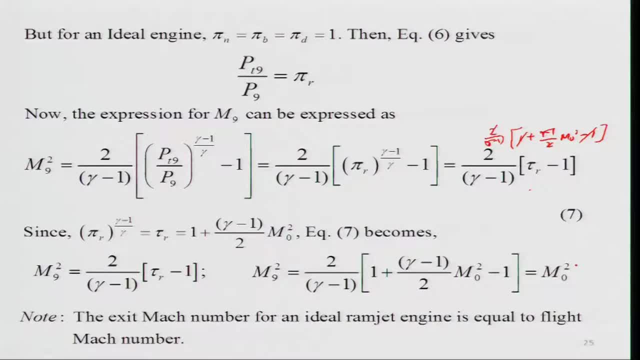 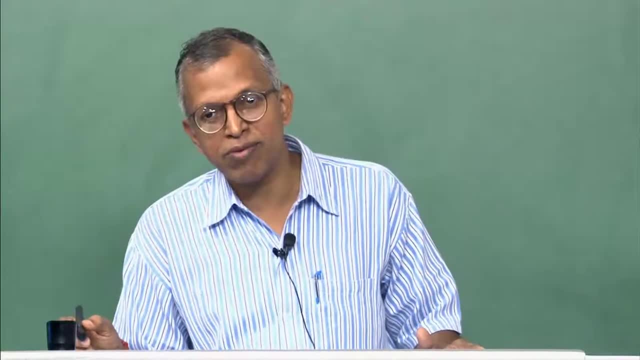 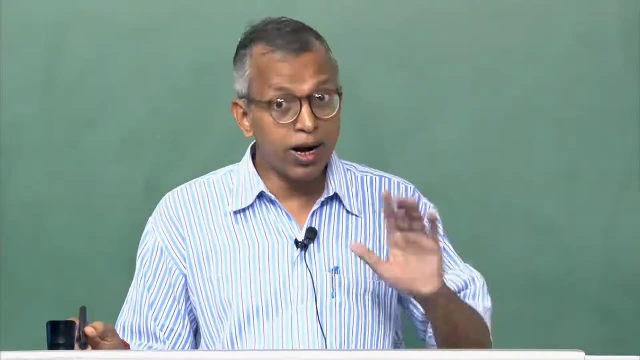 really is happening. that means whatever the velocity of air which will be entering the ramjet, into the ramjet will be same as the exit velocity of the engine. certainly no, it is the Mach number which is same under ideal condition, real situation. it would not be right. 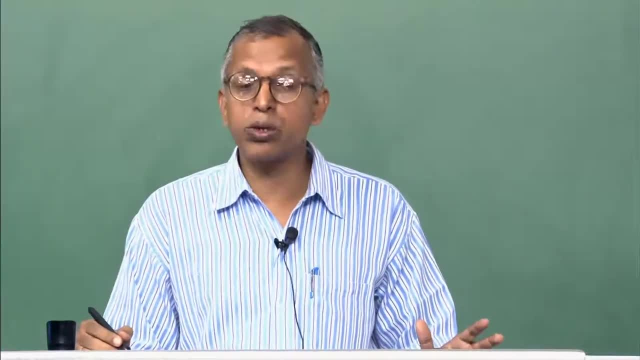 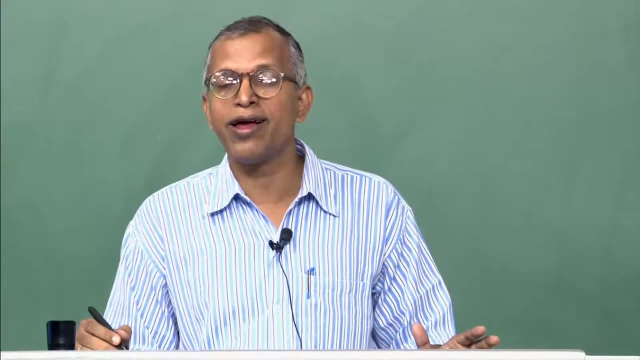 So that is the interesting part. how is here? but you should not assume that exit a nozzle, exit velocity v 9 is equal to the v naught or the flight velocity. So that is another deep probability. 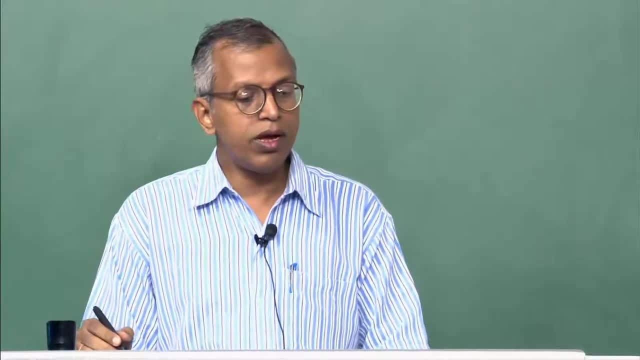 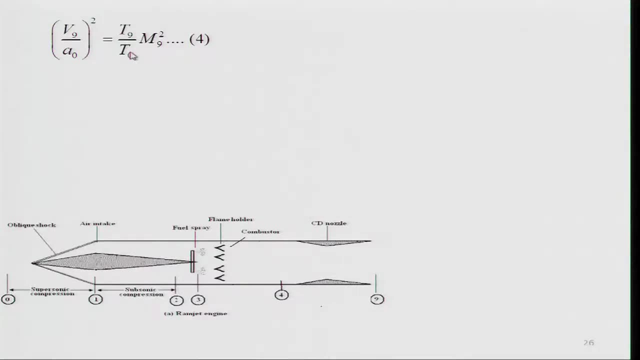 we can say this: T T 9 by T naught, and keep in mind this T T 9 by T 9 will relate to what? 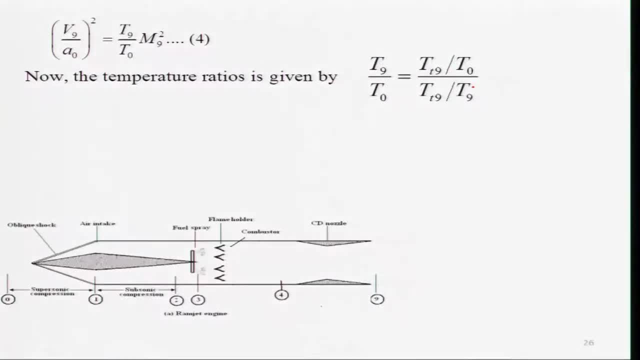 Pressure ratio. Pressure ratio, temperature ratio- all those things can be related, right, and we will now look at T 9 by T naught. in terms of temperature ratio, I can write down: T- T naught- T T 9 by T naught is equal to T T 9 divided by T T. 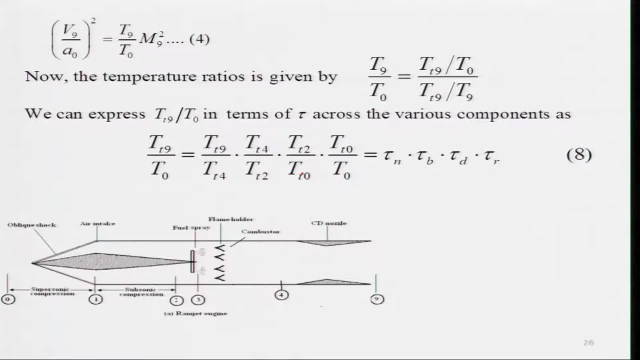 8 into T T 4 by T T 2 into T T 2 by T T naught, T T naught by T naught, right. So if you look at this is temperature ratio what is happening, right? this is nothing but your. 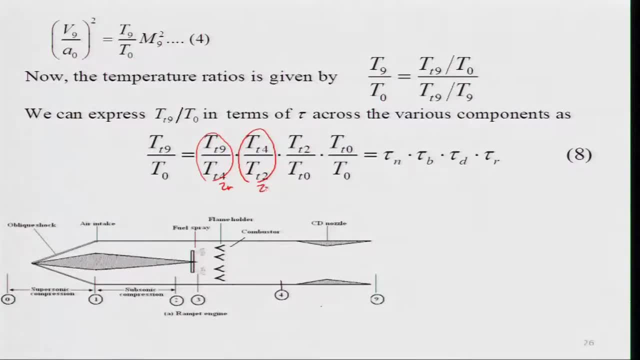 this portion is nothing but your tau n. this is nothing but your tau b. this is nothing but your T T 2 by T naught tau r tau d, and this is of course the tau r right. But if I look at this, can I say that tau n is equal to 1 total, because we are not adding 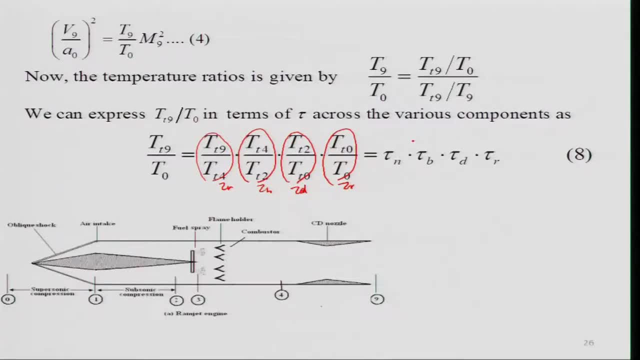 any heat, nor you are taking any heat out of it. adiabatic condition: isentropic expansion: right. So therefore I can say this is 1. can I say that tau b is equal to 1, right? can I say No, sir? 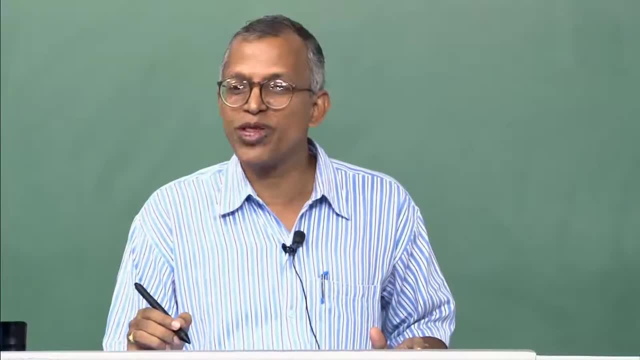 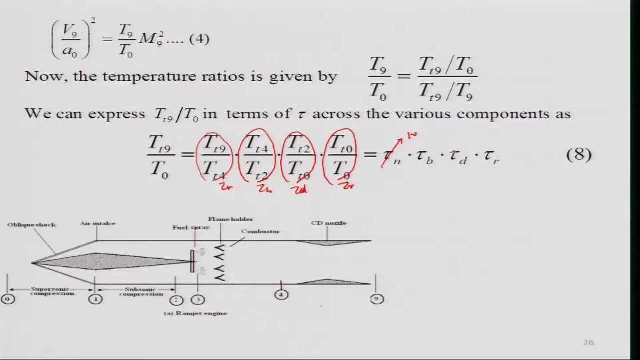 I cannot. I am adding heat right. So therefore the total temperature ratio is equal to 1. ratio across the burner or the combustor cannot be 1, whatever. tau d, I can say: it is Constant 1, not constant 1. ratio is 1 right, and so therefore I will. and tau r, can I say? 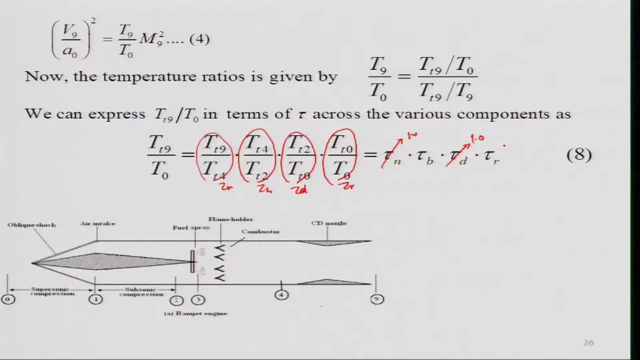 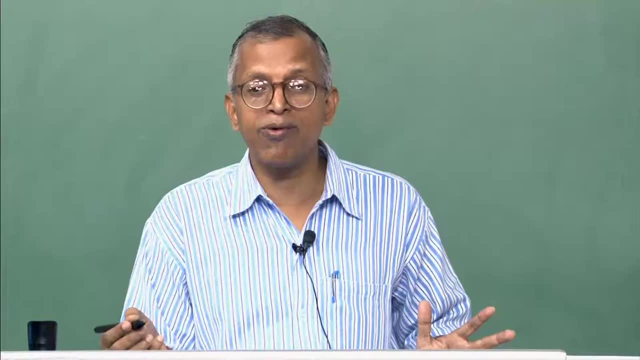 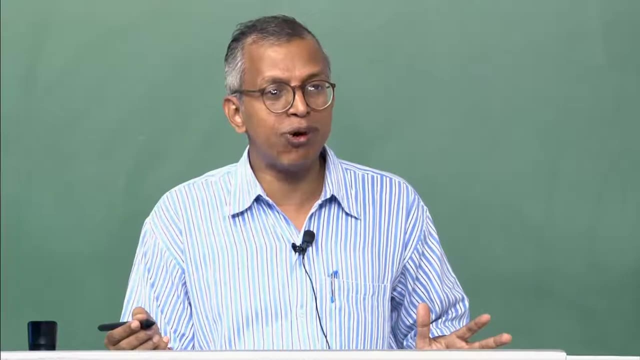 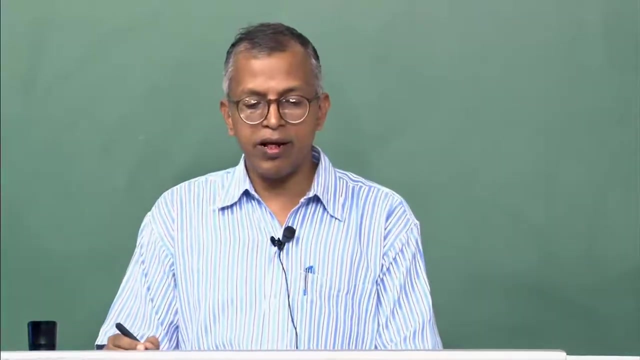 it is equal to 1. certainly no right, because it is the flight dependent on the flight Mach number, right. It can never be 1, it will be more than 1, always, unless otherwise flight Mach number is 0, there it will be 1 right. So therefore I can say: 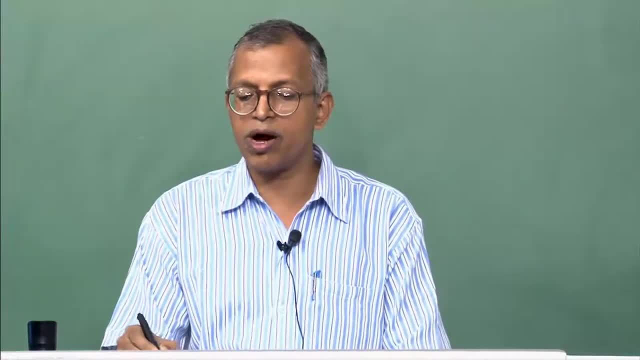 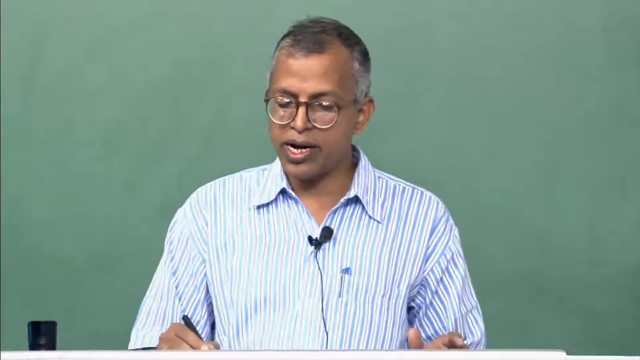 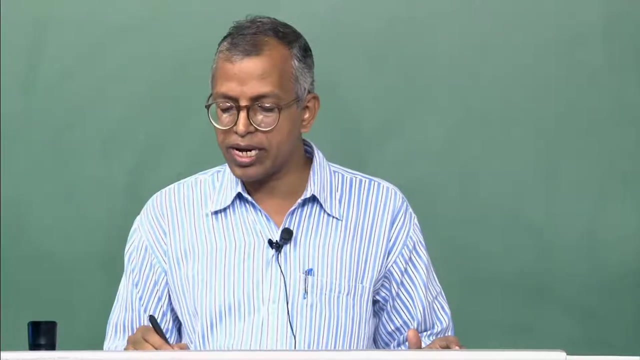 that T 9 by T naught is nothing but tau. b dot. tau, that means multiplication. basically in this case I have used So T 9 by T naught is nothing but T T 9. divide by T naught right and T T 9 by T 9, if you look at that is equal to tau. 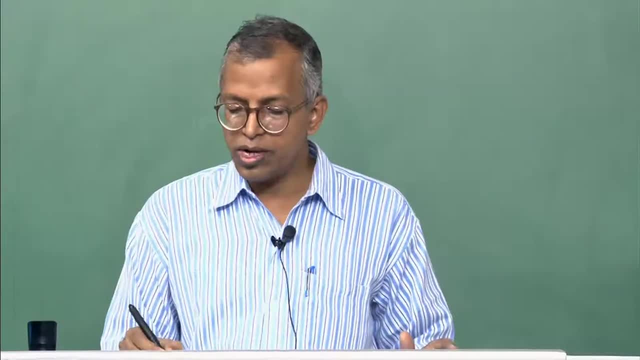 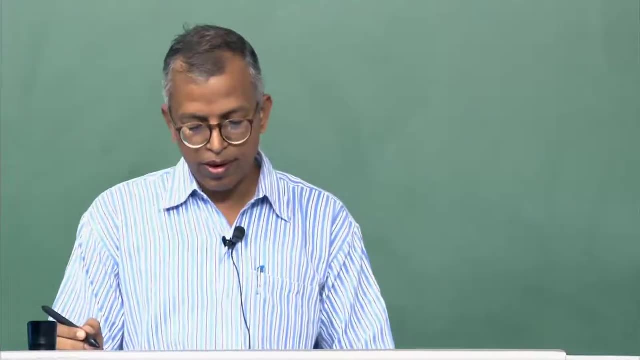 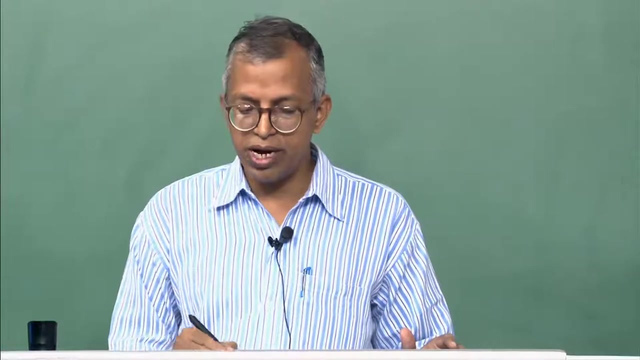 So tau r. we have already seen that earlier, So it will cancel it out. you will get tau b. that means T 9 by T naught is nothing but tau b. and of course- this I have already told you earlier that how it is- T T 9 by T 9 is nothing but your pi r gamma minus 1 there. 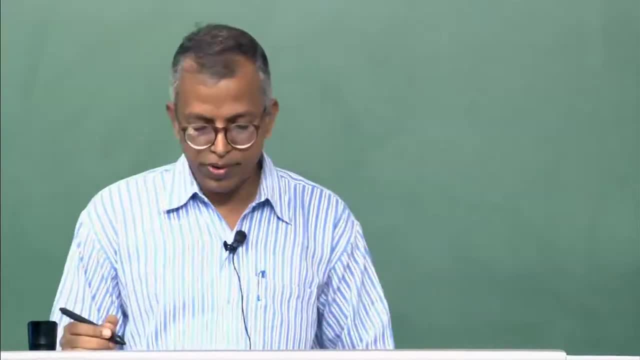 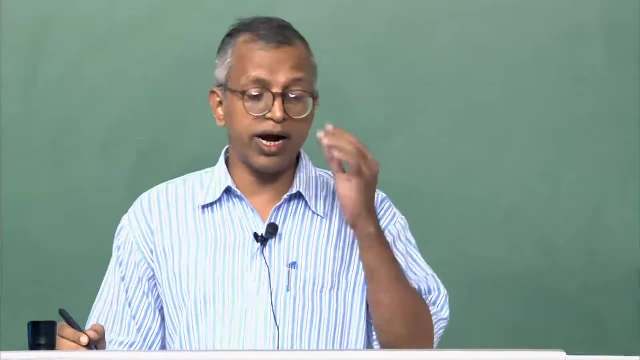 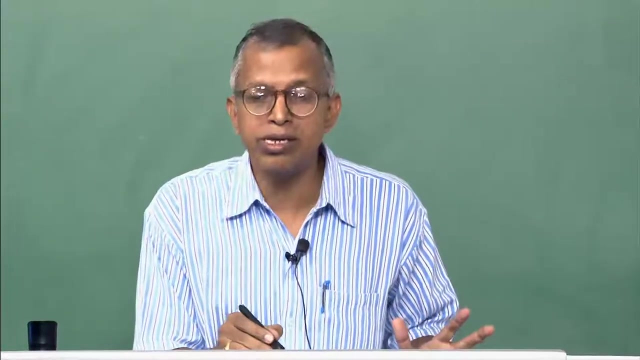 is nothing but your tau right. We have already derived this thing, So we need not do that, we need not to repeat it. So now we will have to look at the combustors and keep in mind that we are assuming the in the this combustion chamber, the flow to be 1 dimensional. 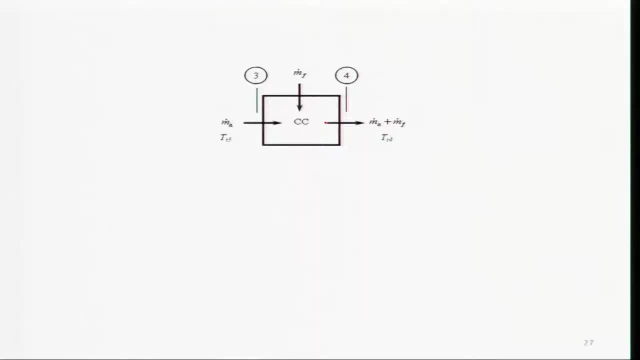 but in real situation it cannot never be And we are assuming that certain amount of air is entering and fuel being added and it is going out with certain mass flow rate of air and fuel, So we can carry, you know, like considering the flow to be 1 dimensional and steady flow. 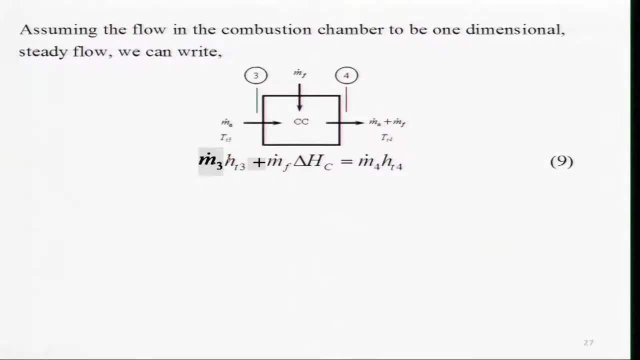 that always we are assuming in this, in analysis, which I think I did not mention- that is the steady flow, And even in real cycle we will be assuming the flow to be steady that you keep in mind. So therefore it will be m dot 2 s T T 3 minus m dot f. delta s t is: 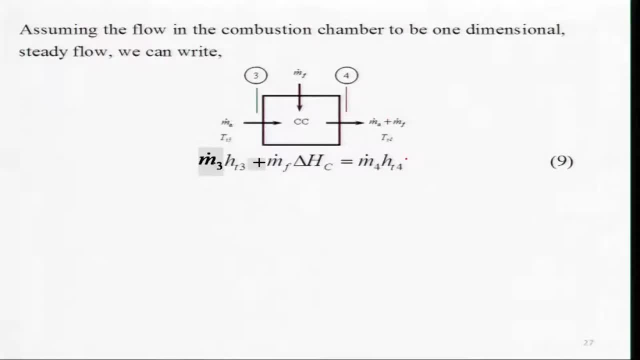 equal to m dot 4 s T 4.. So we are assuming here that continuity equation. you know that m dot 4 is equal to m dot f plus into m dot 3, and we are saying m dot f in this equation particularly less than. 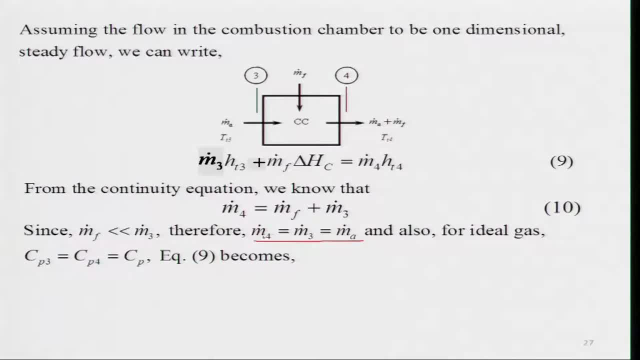 m dot very, very small. So therefore we are saying that is m dot 4 is equal to m dot 3 is equal to m dot air- how much air is entering, And we are assuming calorific warfare to gas. so therefore C p 3 is equal to C p 4 and C p. 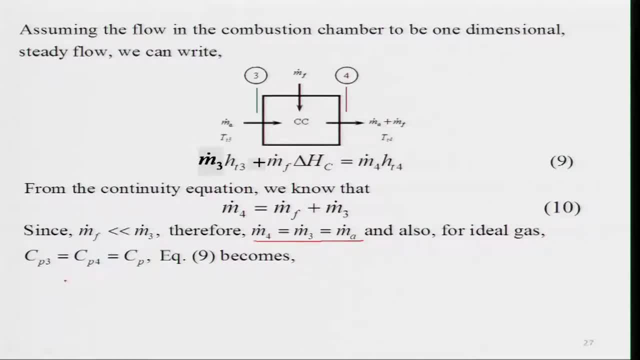 So if I look at this, if I can write down this expression, I can write down m dot equation 9. I am writing C p T 3 plus m dot f, delta, s, c, that is the heat of combustion, m dot a and C p T T 4. right, If I could write this expression? for the simplify what I will write. 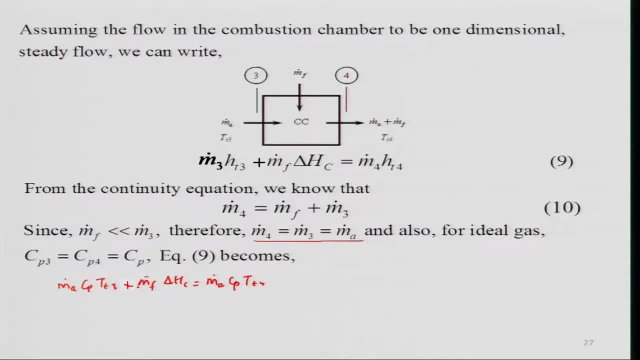 What I will get. I will get m dot f, delta s, c is nothing but m dot a C, p, T T 2, because T 3 is equal to T T 2, right? So in this place I can write down: you know, T T 3, T T 2.. So 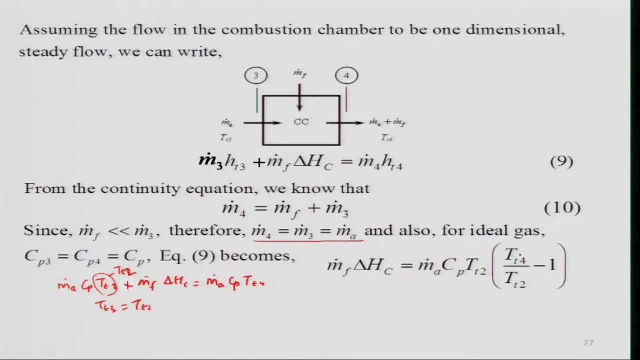 I can take this out: m dot a C p, T T 2 and T T 4 by divided by T 2 minus 1.. So what I can write down here basically: m dot f, delta s c is equal to m dot a C p right and T T 2. 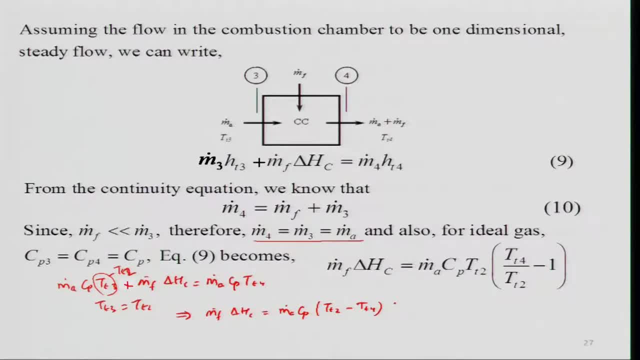 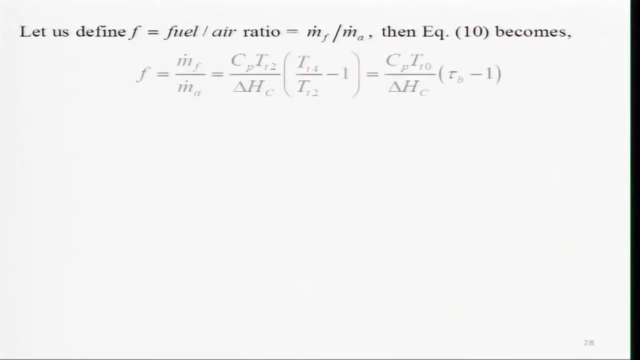 minus T T 4 and I from that I can get this, like if I take T T 4 out. no, no, sorry, there is some problem. T T 4 minus T T 2.. So if you take this out, you will get T T 4 by T T. So let us. 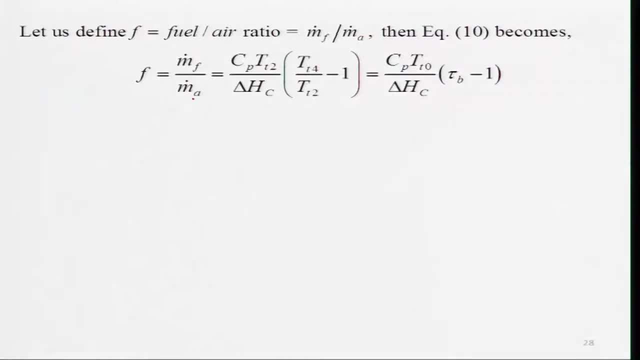 define: f is equal to m dot f by a, and then from that expression I will get: m dot f divided by m dot a is equal to C, p, T T 2 divided by delta s. c is T T 4 divided by T T 2, and this: 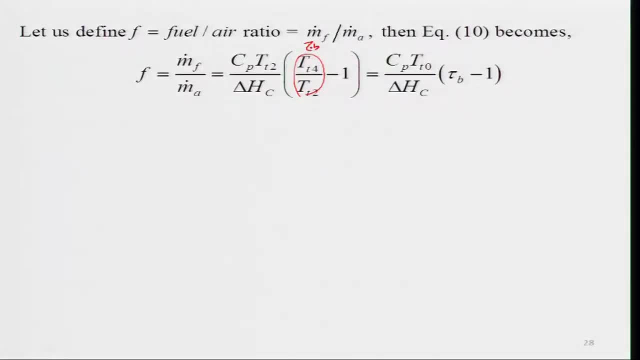 is nothing but your tau T T 4 plus tau b, by definition right, because we are assuming T T 2 is equal to T T c. there is no, you know, compression here. So therefore we are, and keep in mind that this T T 2 will. 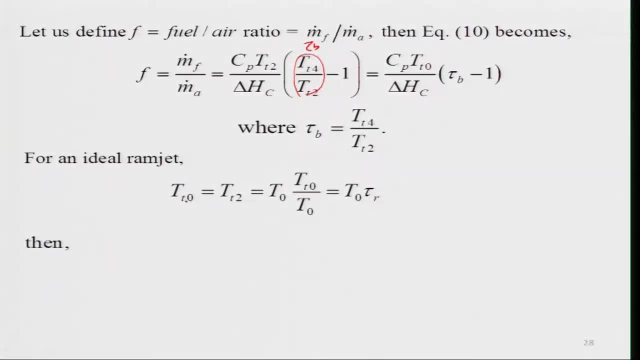 be same as T T naught, right, because T T naught is equal to T T 2 and no heat being added, as shown in the what you call T s diagram. So therefore I can write down T T naught by T naught and this, by definition, is nothing but tau r. So T naught by tau r. Then we can. 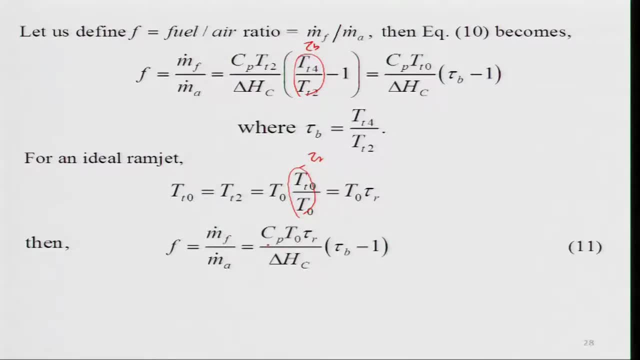 write down as: f is equal to m dot, f by m dot a is equal to C, p, T, naught, tau r, delta s, c, tau b minus 1.. So now we shall write down basically the one definition which we will be using. I did not define. let me define that. 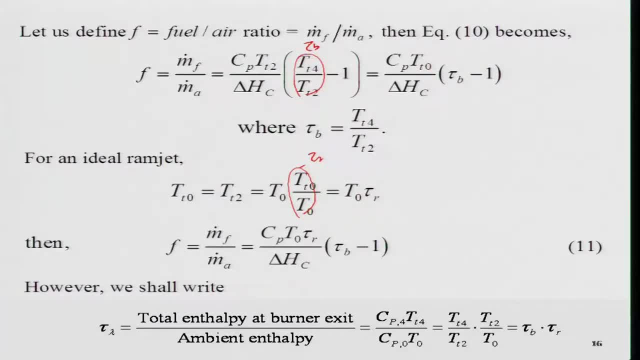 is a total enthalpy at the burner exit, that is, you can say it is a- this is a little mistake here- So 4 and T 4 and this is not required. So T, T 4 by T, T 2 and T 2 by this. So will. 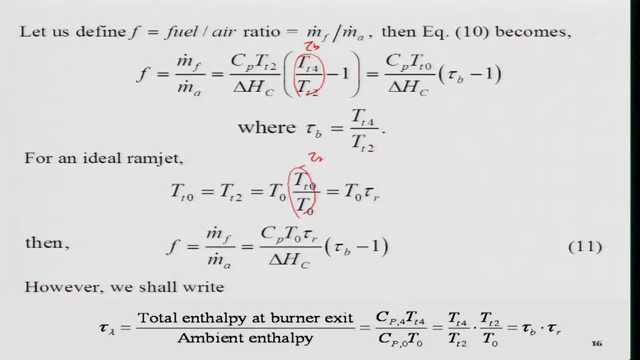 be tau b into tau r right. The total enthalpy at the burner exit right will be C p 4, T, T 4. divided by this thing: C p naught by T naught, So that I can say that C p, C p, this will. 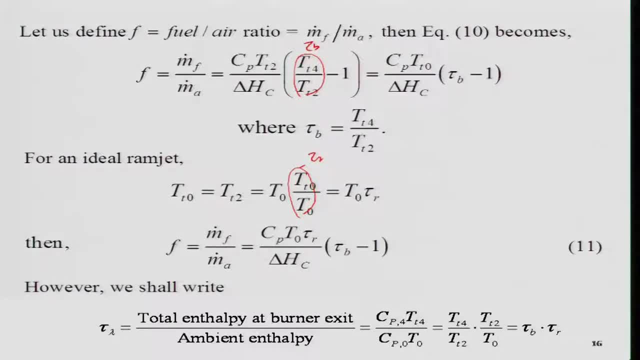 cancel it out. So therefore, T T 4 by T T 2 is equal to T T 2 by T naught, equal to tau b by tau r. That means what you are saying tau lambda is basically tau b tau r. right, and this will be using you know some places, So coming. 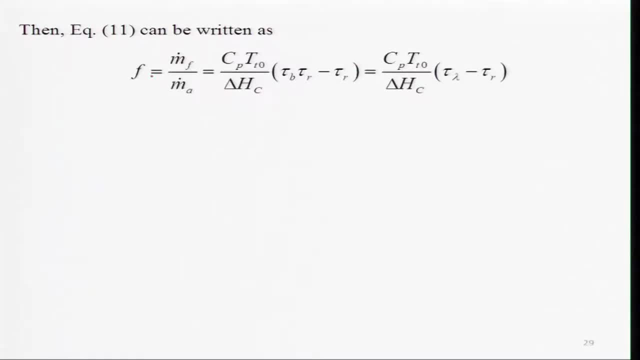 to that, like I can write down. you know this F is equal to m dot, F, C, p, T, naught delta S, T, tau b tau r. I can write down tau lambda right and minus tau r, So V 9 by A naught square. if you look at what we have done, 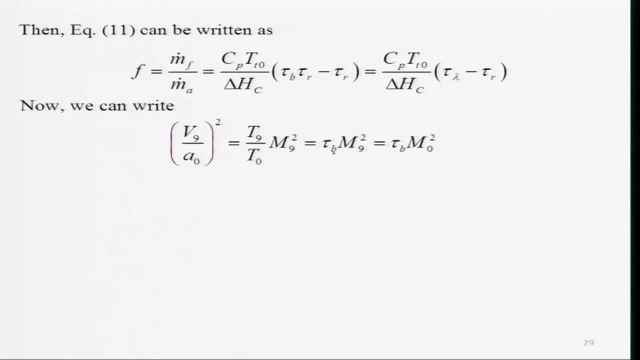 We have find out T 9 by T naught m 9 square and this is nothing but your tau b and m 9 is nothing but your m naught square. So that became tau b, m naught whole square. So then, 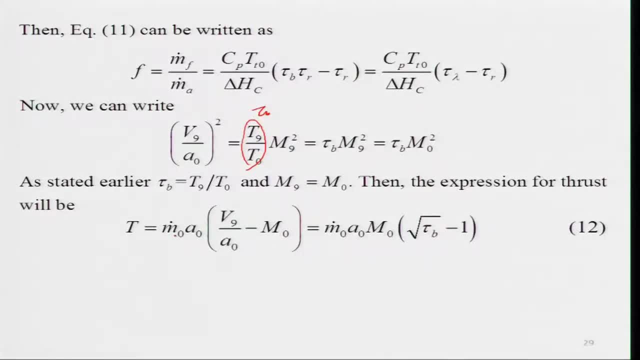 our expression for the thrust. if you look at it will be in this place. what will be using is basically root over tau b m naught. So if I take this m naught out, it will be m naught A naught square, m naught root over. 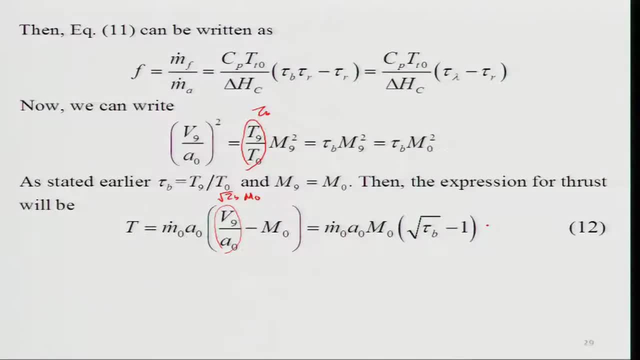 tau b minus 1.. This is a very, very simple expression. what it says to you? it says the thrust will be dependent on the amount of mass flow rate entering into the engine. It will be dependent on also the flight Mach number and it will be also dependent on tau. 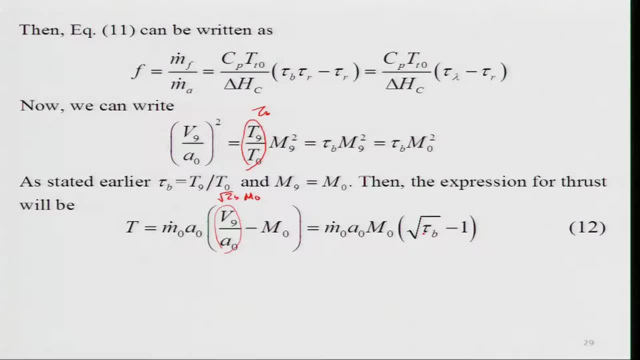 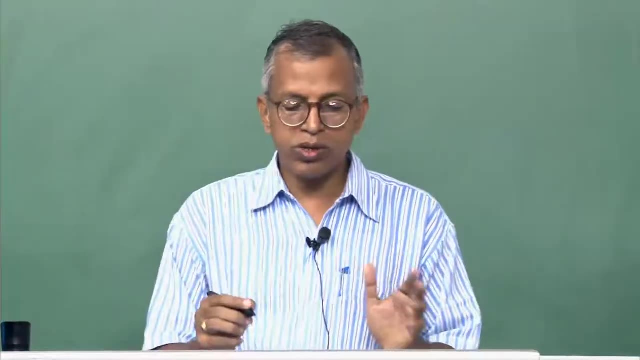 b, that means how much energy you are being added. tau b will be representing temperature ratio across the burner, which will be dictated by how much you know fuel you are being burned, So that total temperature will increase, right? So this is the simple expression we are getting. 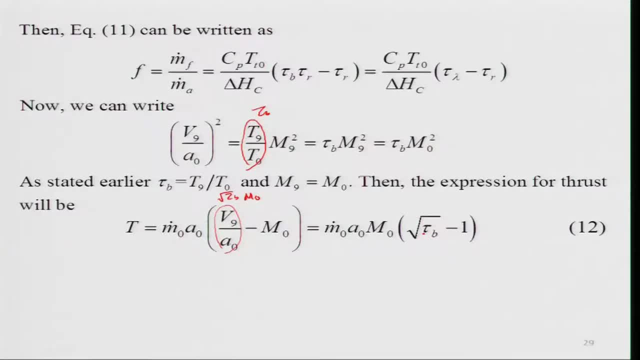 and we will be varying this parameters and see how it is, you know, dependent on what and what are the conclusions. So that is why call it as a parametric segment, rewriting equations to get a specific, you know, get a specific thrust, because if I just divided by m dot A, here m dot A or m naught. 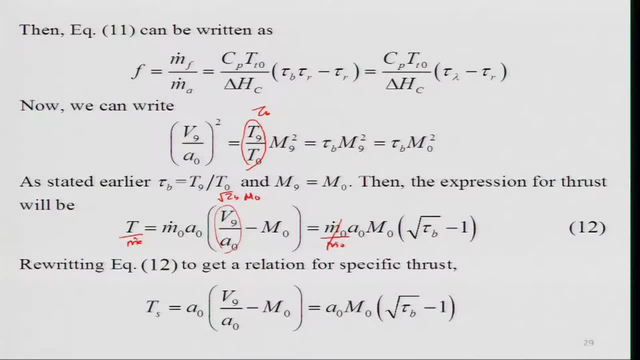 So then I will get specific thrust a naught into V 9 by n r minus m naught, so that you can write down m naught root over tau b minus 1.. Next one: Basically the same thing, only this is the specific thrust and that is the thrust So. 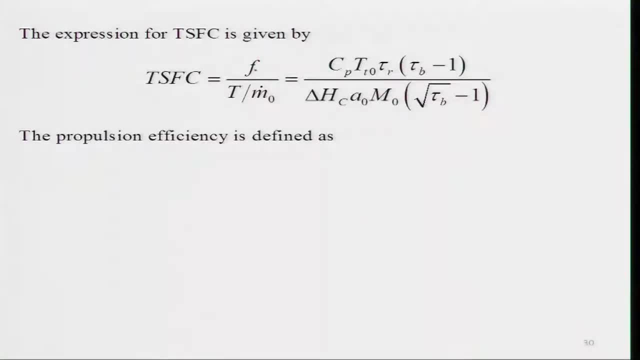 now what we will do. we will look at T, S, F, C. just you know, put these values F and then specific thrust you will get. there are several terms are coming into pictures and of course it is a function of similar stuff, except the delta. S, C has come into pictures, right? 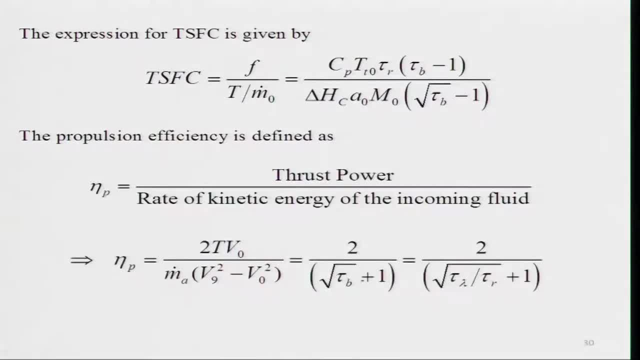 And propulsive efficiency will be. you know you can express in terms of tau v, right in place of tau v. you can talk about tau lambda by tau r, because tau v is related to tau lambda, or tau lambda is related to tau v and tau r. we know that tau lambda is equal to 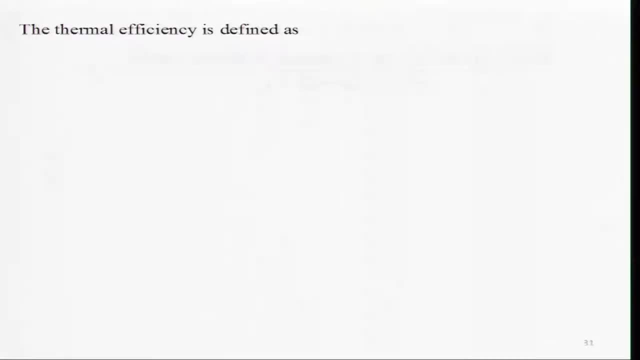 tau v tau r And if you look at thermal efficiency it will be similar. you can note that the thermal efficiency is equal to 1 minus tau r. That means it is dependent on the, only on the flight Mach number. it is not dependent. 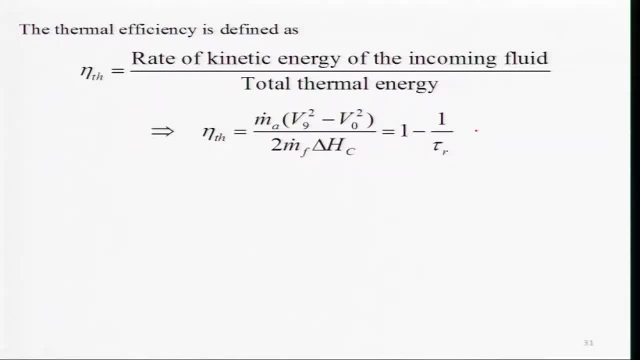 on tau v and other thing like how much heat being added, is not really this thing. that is a very interesting result. right And overall efficiency, of course, is a multiplication of that which is dependent both on the tau r and tau v, because tau lambda when I am saying